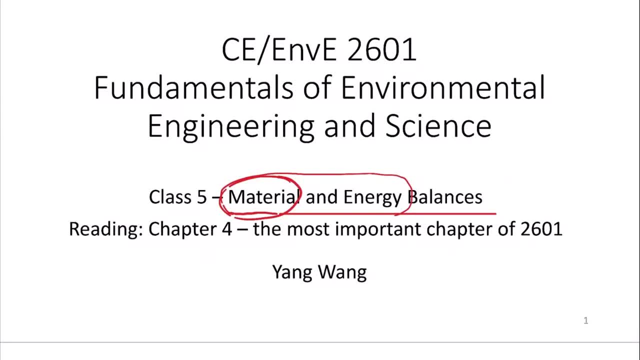 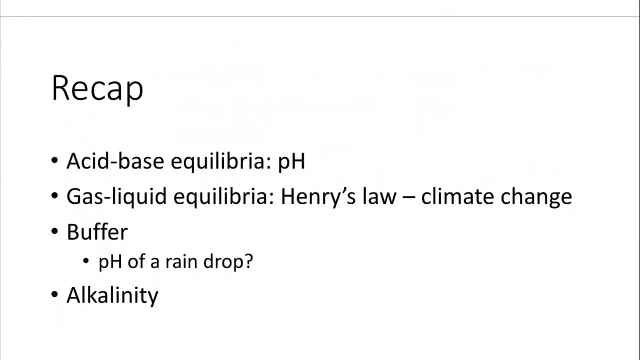 the basic chemical concepts we have gone through so far, And later on you will realize, actually, how we're going to use these concepts in solving the problems. Okay, So please use your time to read this chapter as well. I think it's going to be very helpful, So let's do a. 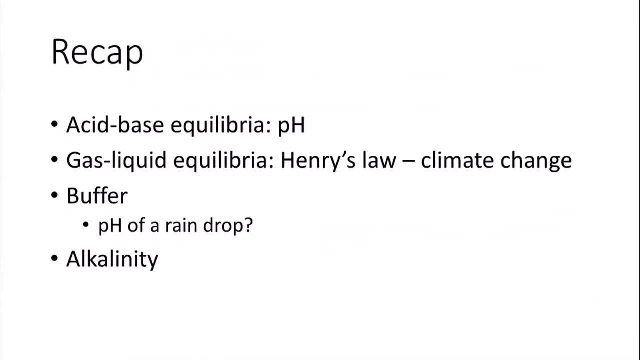 quick recap of our last class. So last class we spent quite a lot of time talking about the acid-base equilibria. or, more importantly, is the pH right? So the pH is basically we're applying this parameter p as a calculator, right? So pH is just negative of log 10,. 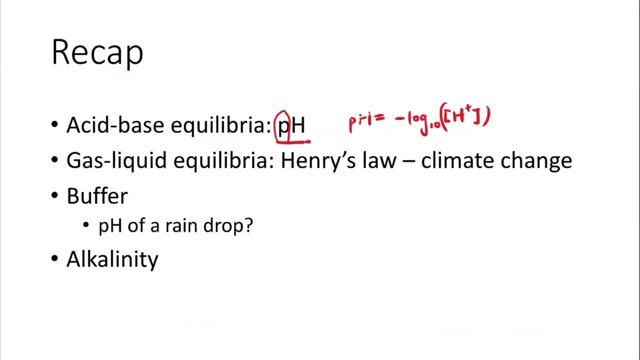 the concentration of hydrogen ions. Okay, so a pH equal to two means that, okay, we've got a pH of 1.2,. hydrogen ion concentration is 10 to the negative. two m or mole per liter. okay, so you don't have any coefficients or two or something else in front of this value here. 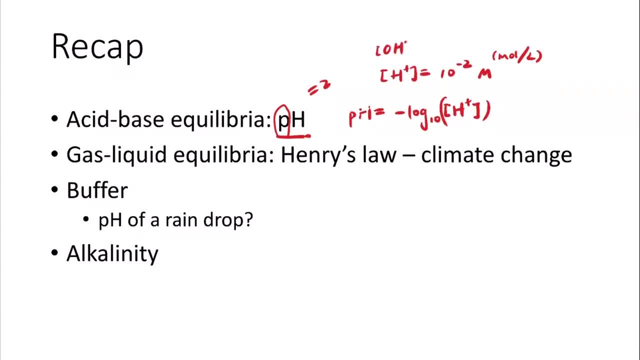 so, based on the pH, we can also calculate the OH ion concentration. all right, so that's going to be 10 to the negative, 14 minus 2. okay, it's 10 to the minus 12. yeah, so this is because we know that the k water, or the equilibrium constant for water, is: 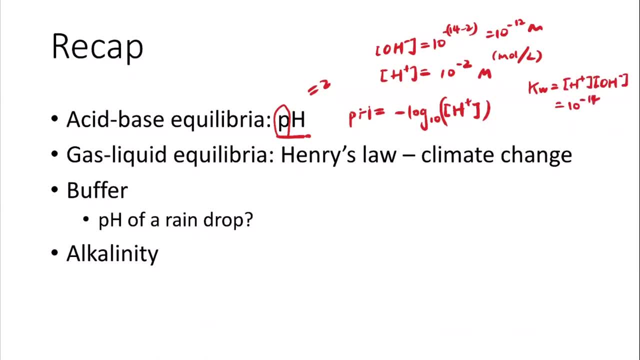 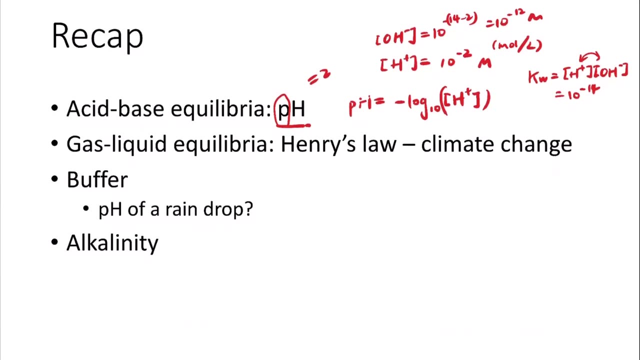 is 10 to the negative 14.. okay, so this is what people derived in their experiments. so if we know any of these ion concentrations so we then can solve, solve the other one in this, I would say this: couple of ions. okay, so we also talked about the gas liquid. 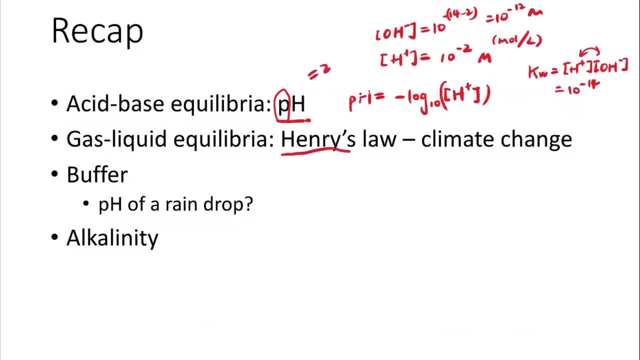 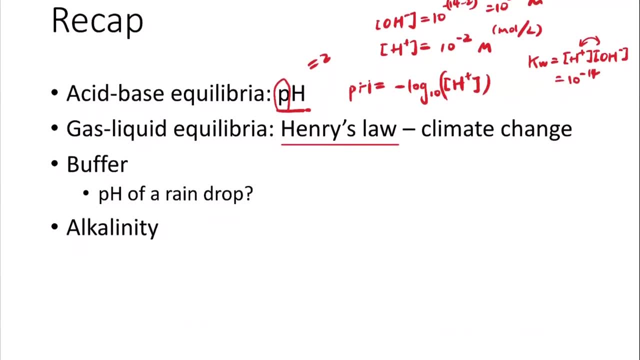 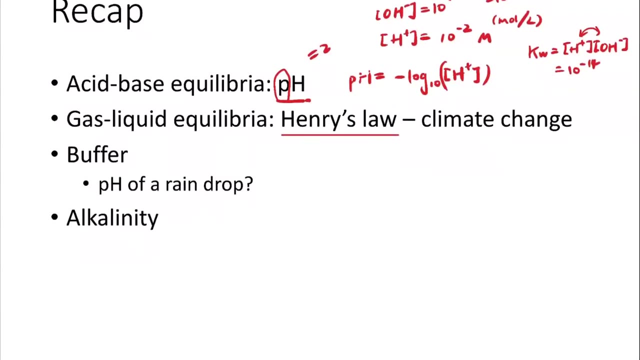 equilibria. so more specifically, it's about the Henry's law, right? so we were saying that the if you know the pressure of certain gas over a liquid, then you can also calculate what is the concentration of the gas within the liquid. so we said this is very important. 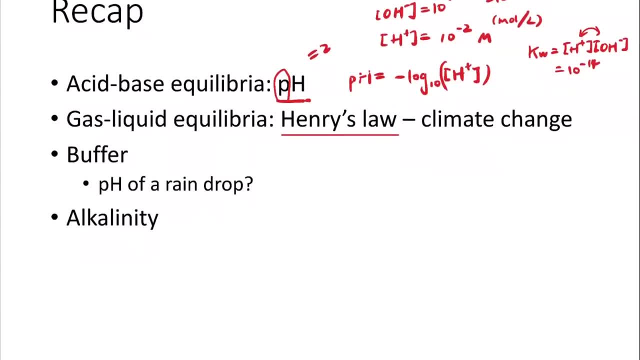 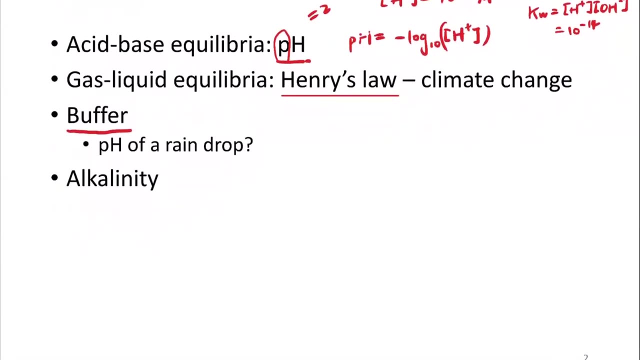 for the climate change because the carbon dioxide has a very low Henry's constant. so that's why most of the emitted carbon dioxide are in the gas or are in the atmosphere, and that's causing the global climate change. so we also talked about the buffer system. so the buffer system is a system of ions or a solution. 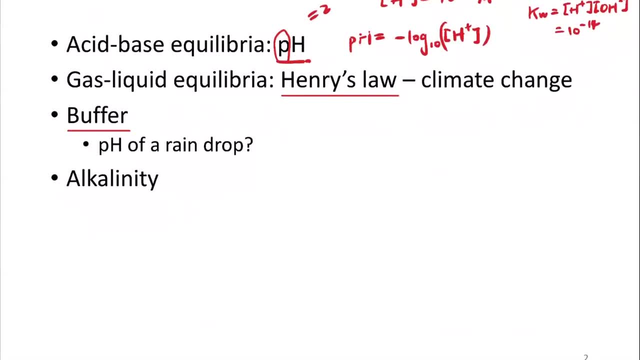 that can withstand a large change of pH, right? so, instead of changing the pH from seven all the way to one, right, when you have these carbonate species, you don't have the excess hydrogen ions and you can. basically, the pH change will be smaller when you pour these strong acids, or. 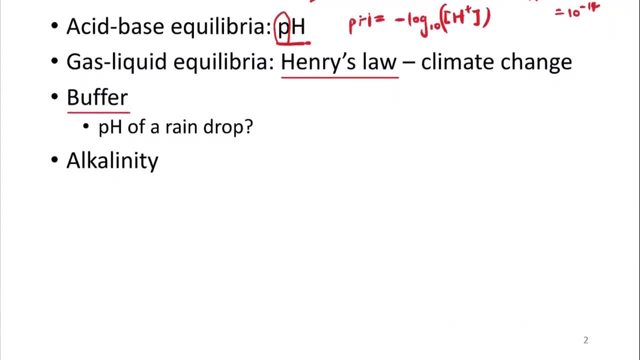 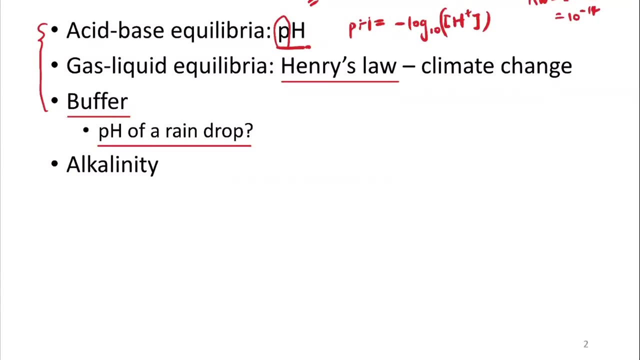 base into the solution. so, with these concepts, we also briefly went through the process for calculating the pH of a raindrop. right, it says it's using basically using all of these concepts. so the gas liquid equilibria, the acid base equilibria, right, so we can solve that basically. 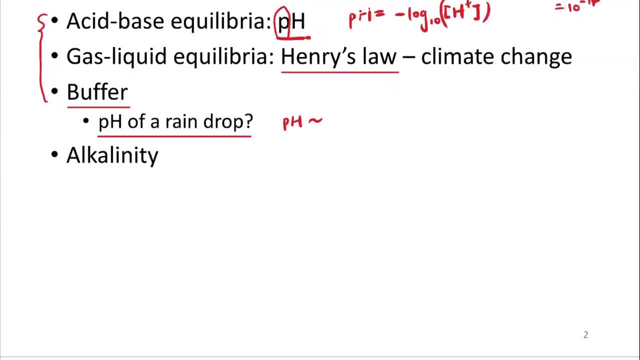 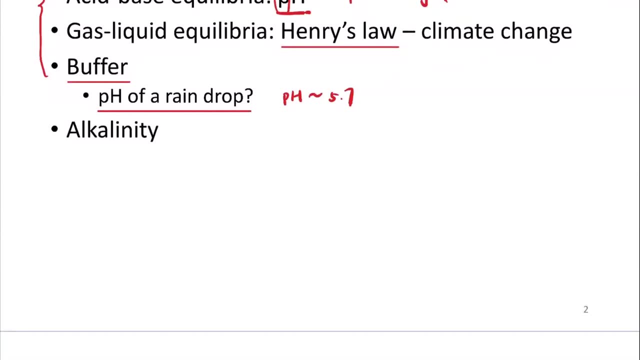 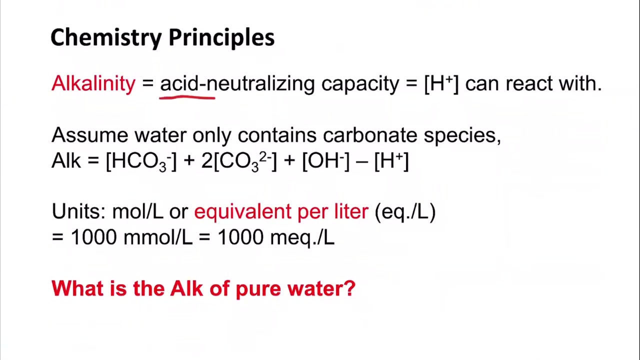 for a raindrop. it's acidic, right, has a pH of around 5.7. so finally, we introduce the alkalinity. so alkalinity describes how much alkali it contains in the solution, or, more specifically, how much acid it can neutralize, right? so if we just finish up this discussion. so the alkalinity is defined as the acid neutralizing. 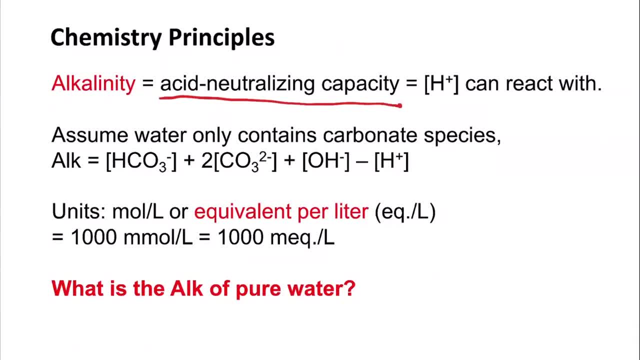 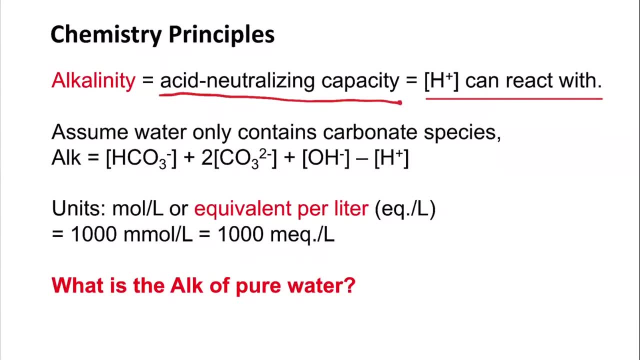 capacity, right. so basically it describes how much hydrogen ions it can react with. okay, So if we assume that the water only contains these carbonate species, let's say the carbonate ion or bicarbonate ion, OH ion and hydrogen ion, then we can calculate what is the alkalinity, right? 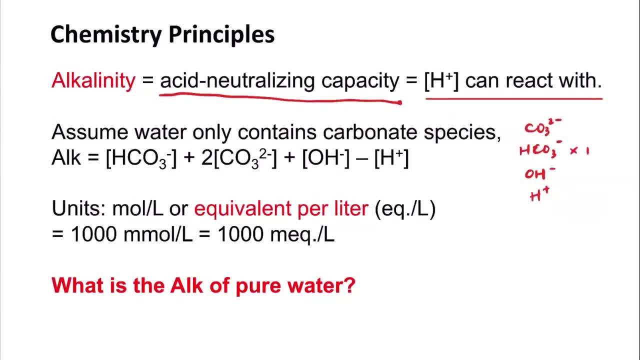 Because we know for each number of the bicarbonate ion it can only react with one number of the hydrogen ion. And then for the carbonate ion, it can react with two number of the hydrogen ion. right For OH ion, it react with one. 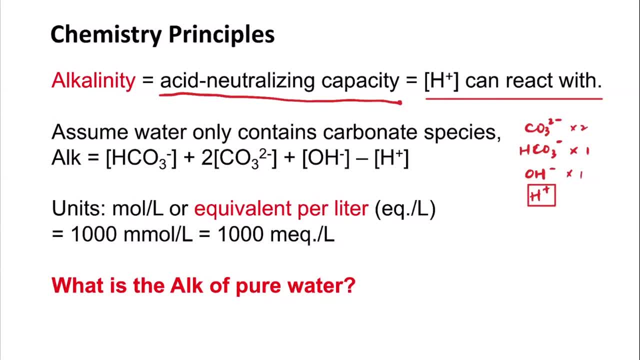 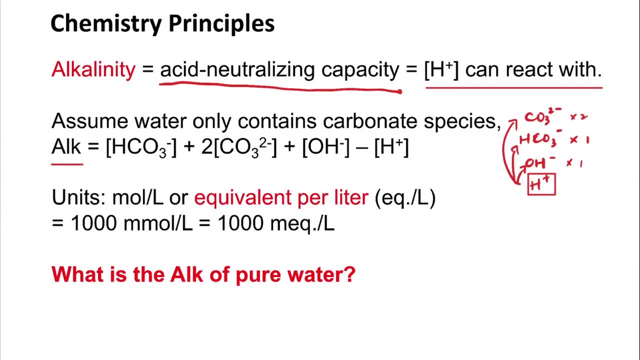 For existing hydrogen ion in the water, then we need to deduct them because they are going to react with these species. okay, So that's why we have this equation here. So the alkalinity, or the ALK, is equal to the concentration of the bicarbonate ion, and then the concentration. 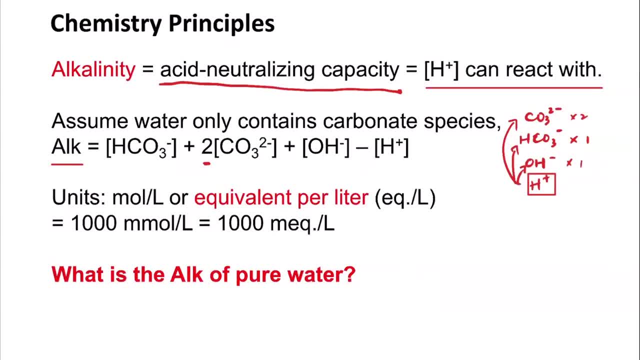 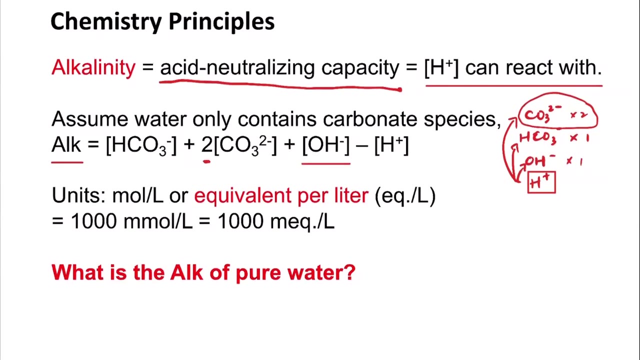 of the carbonate ion multiplied by two, because it's reacting with two hydrogen ions. okay, And then plus the OH ion and then minus the hydrogen ion. Okay, so this is basically the equation that we use to calculate the alkalinity, But we need to make sure that for these units, 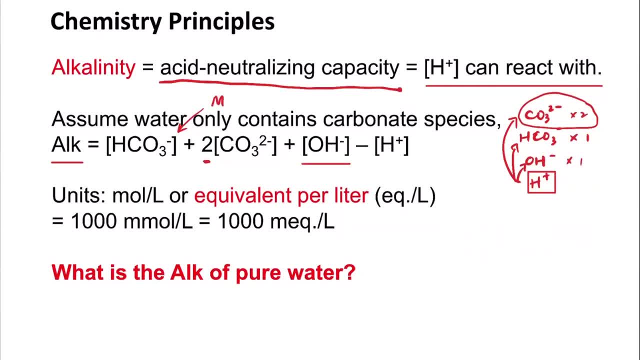 they all have to be in molarity, okay, So basically it should be M or mole per liter. okay, We cannot directly add their mass concentration inside, because we need to basically describe how much hydrogen ions they can react with, right. So we know that each of them have a different. 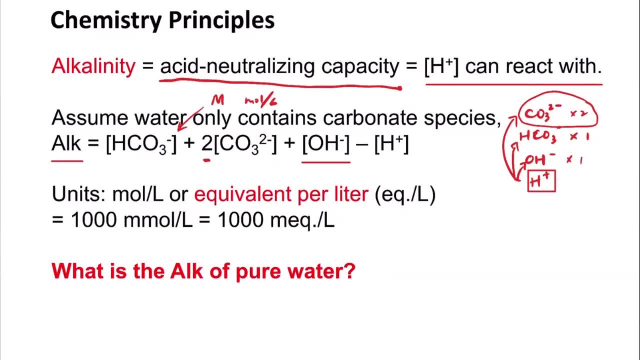 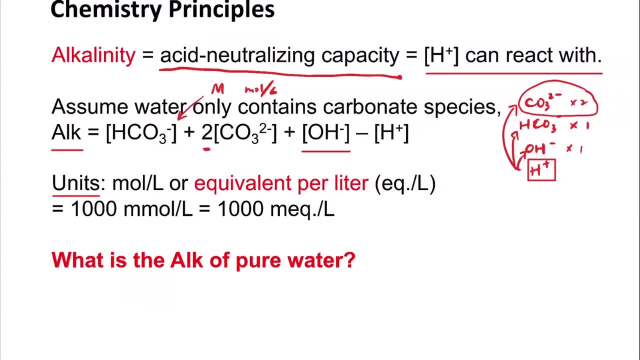 one molecular weight. So we need to convert them into mole per liter first, okay. So that's why, in terms of the units of the alkalinity- okay, they all have to be in molarity of the alkalinity- people can use mole per liter, okay. 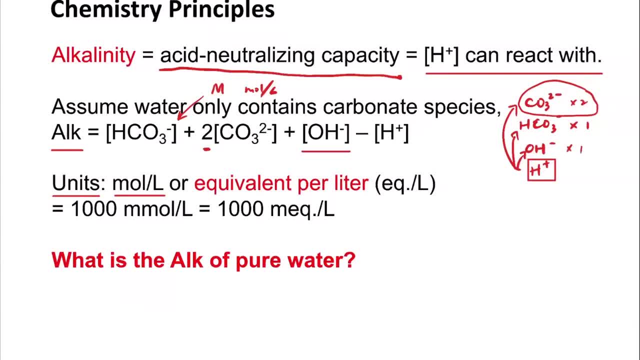 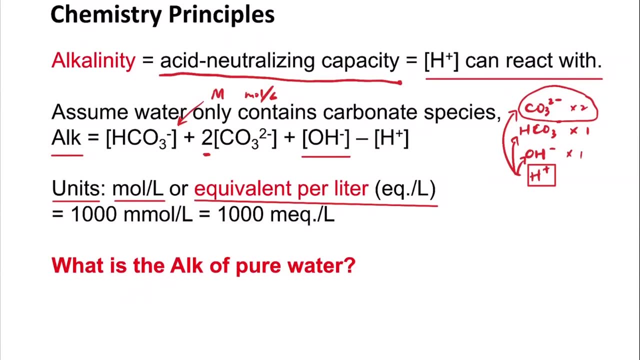 Or they also invented a term called the equivalent per liter. So the idea of using equivalent per liter is that, although it's describing how much hydrogen ions they can react with, but actually there's no hydrogen ions in the water for us to react with it. okay, 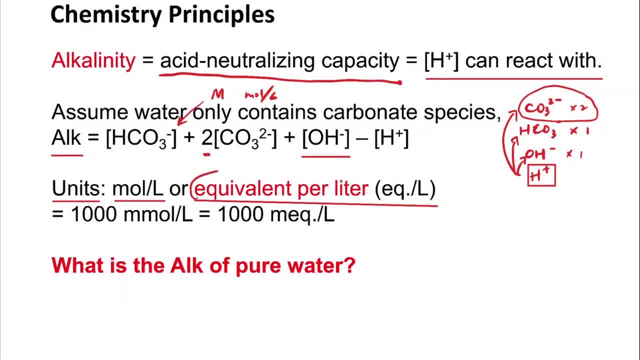 So that's why we call it equivalent. So basically, to show that this amount of carbonate species is equivalent to how much amount of hydrogen ions in the solution. okay, So for simplicity we'll also call it Eq dot per liter. So whenever you see the Eq dot, it just means mole, okay. 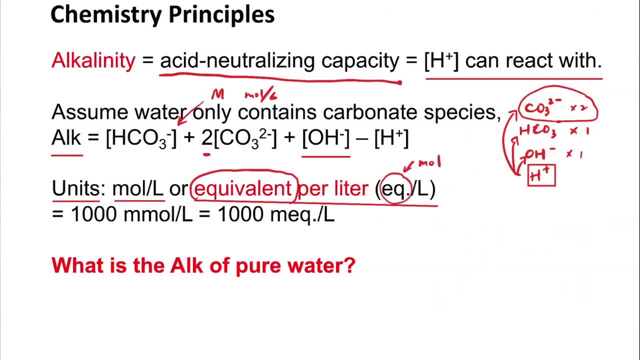 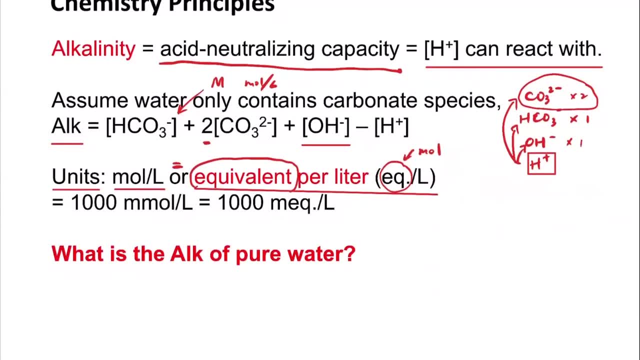 Mole per liter, all right. So the mole per liter is equal to equivalent per liter, And because the ion concentration in the water is normally quite low, so people also will use the unit of millimole per liter. So that's just one thousandth of a mole. 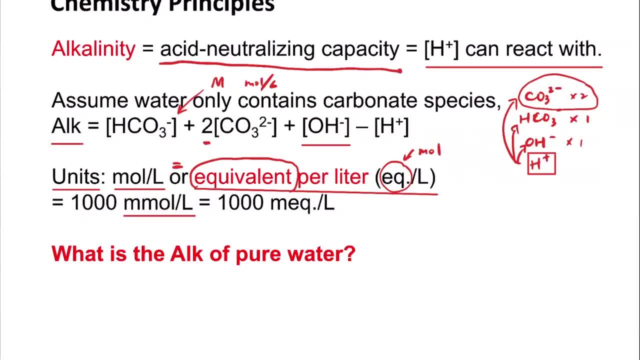 So that's equal to: basically: one mole per liter is equal to 1000 millimole per liter. And also for equivalent- people also came with this unit here- Meq milliequivalent per liter. okay, So it's equal to 1000 milliequivalent per liter. 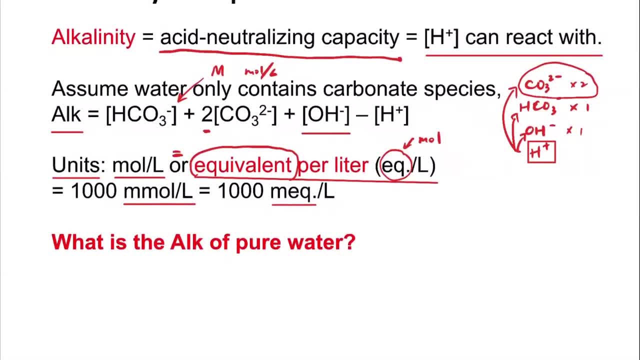 So, based on this definition, if I ask the question, what is alkalinity of pure water? Okay, what's this equation? That water doesn't have any other ions other than hydrogen and OH ion. okay, So what's going to be the pH if I raise this quiz here? 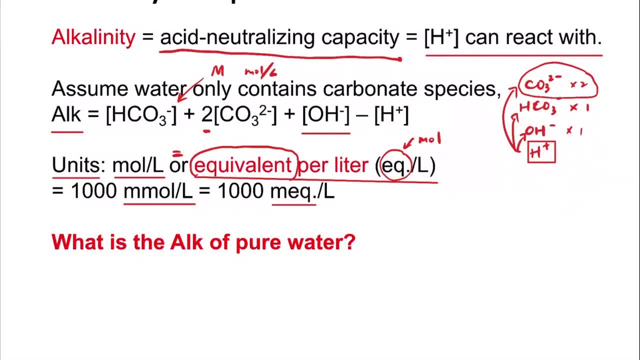 So what's going to be the pH if I raise this quiz here? So think about the difference in the definition between pH and alkalinity. okay, So I saw some of you were choosing the pH. Alkalinity is different from pH. Alright, 10 more seconds. 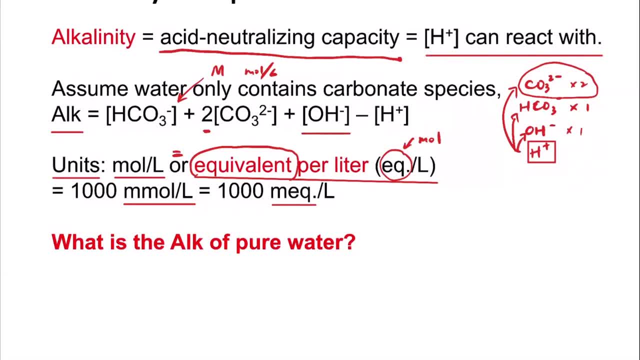 Okay, we'll stop here. I'll share the results. So most of you are correct, but when I see the number pop up, I think, I think or I can answer. I can answer. this is actually another question. at first, many of you chose the 7.. So 7 is the pH. okay, So it's just the concentration of the 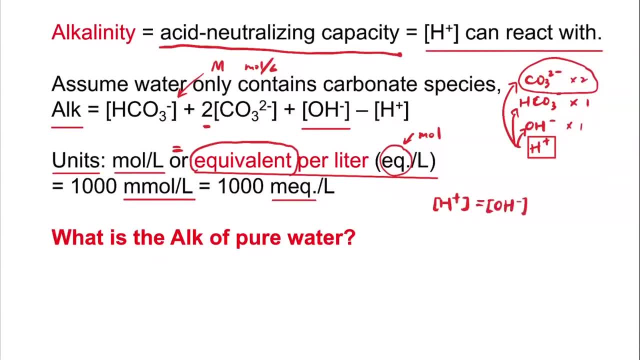 hydrogen and OH ions in the pure water is the 10 to the negative 7, okay. So that's why pH is equal to 7, because you just take negative log of 10 of the hydrogen ion concentration. okay, So if you plug this in, that's going to be 7, all right, But this is pH. So here we're. 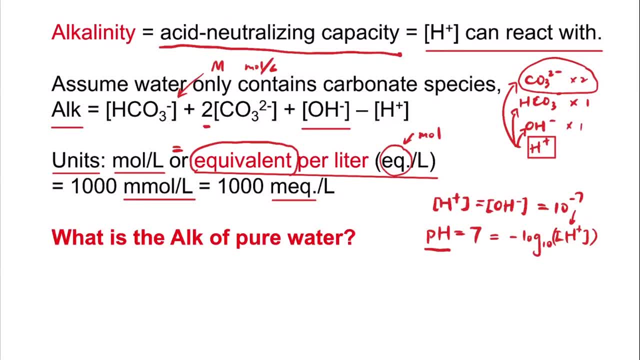 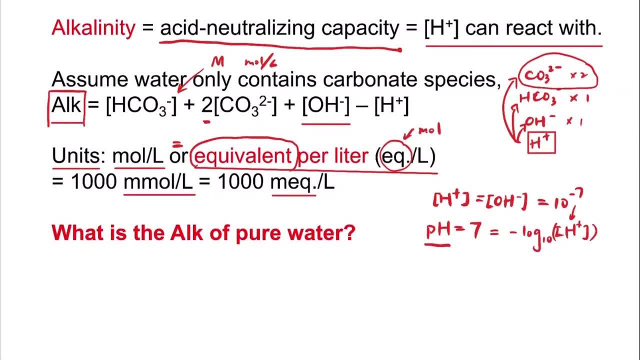 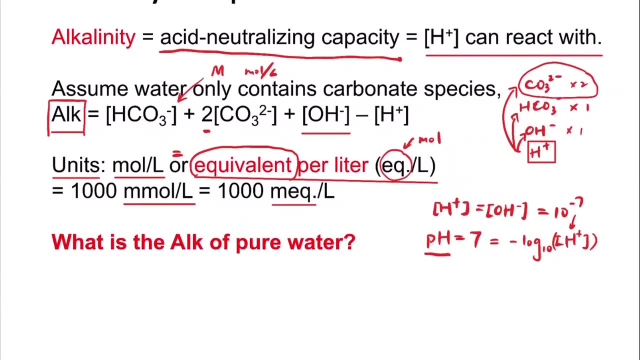 talking about alkalinity. So when you calculate the alkalinity you plug in this equation. So it depends on the concentration of the bicarbonate ion, carbonate ion, OH ion and hydrogen ion. So we said this is pure water, right? Pure water doesn't have any. 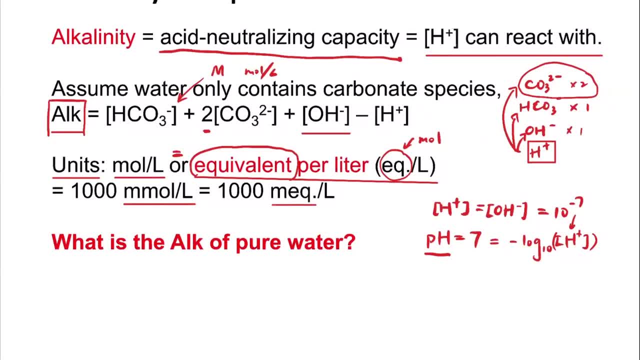 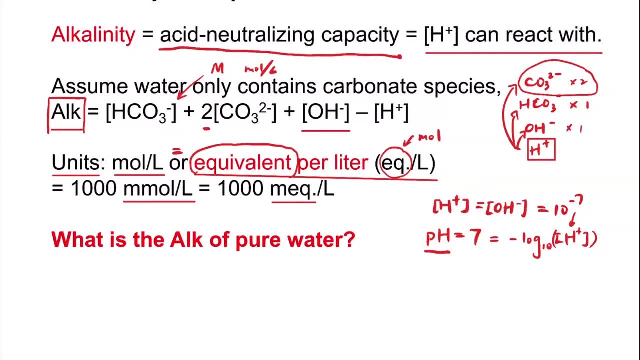 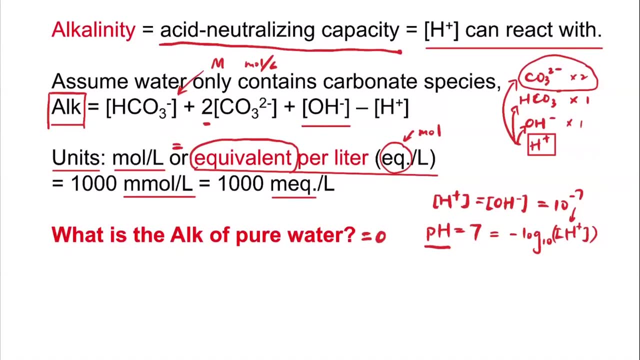 carbonate species. So it's just hydrogen and OH ion, And we know that for pure water the concentration is the same, right? So basically, it's just the 10 to the negative 7, minus 10 to negative 7, and you will get zero here. okay, Let me know if you have any questions. 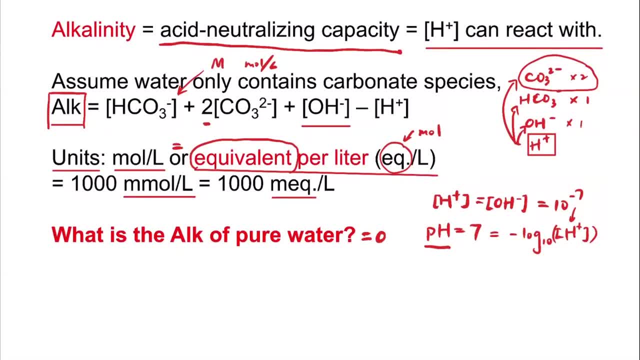 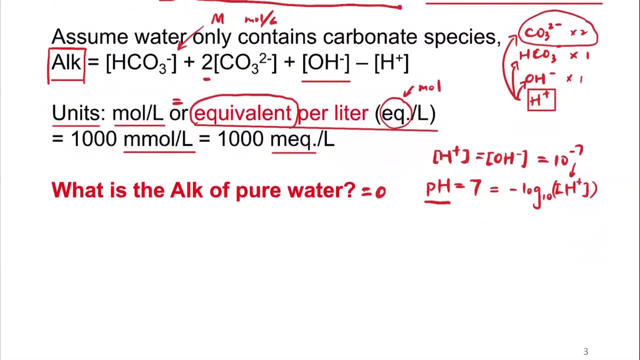 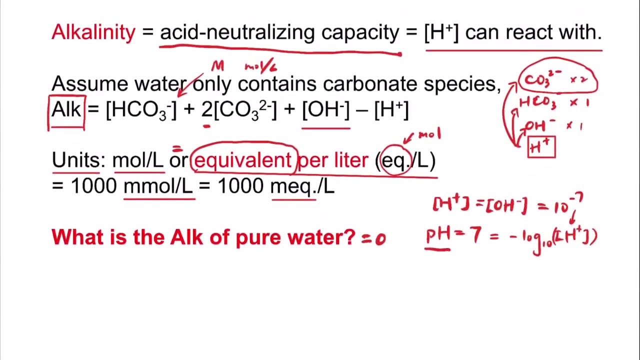 about the concept for the alkalinity, or pH. I really want to make it clear so that later on, when we see water treatment or when we design water treatment or wastewater treatment system, we need to use these data. Okay, So I would say this is a quite simple example solving the alkalinity. This is directly 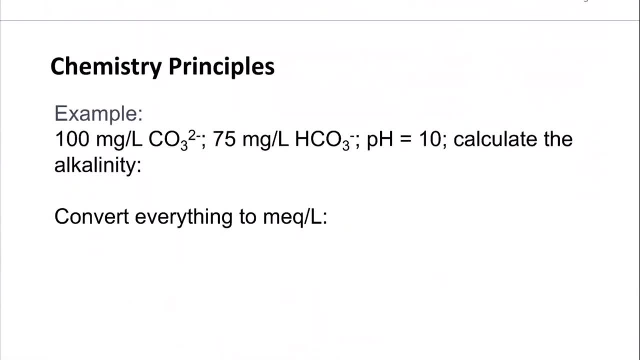 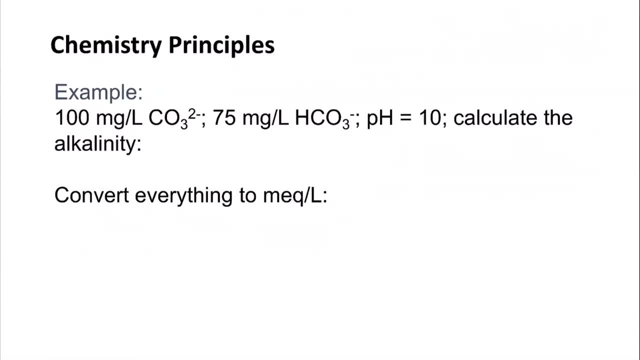 equal to zero. So what about a real water sample, which we need to really calculate the alkalinity? Okay, so let's spend several minutes so that you guys can spend some time on this question. okay, So let's say we have a solution that contains: 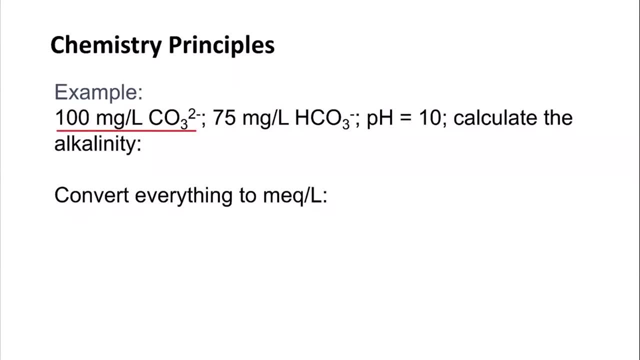 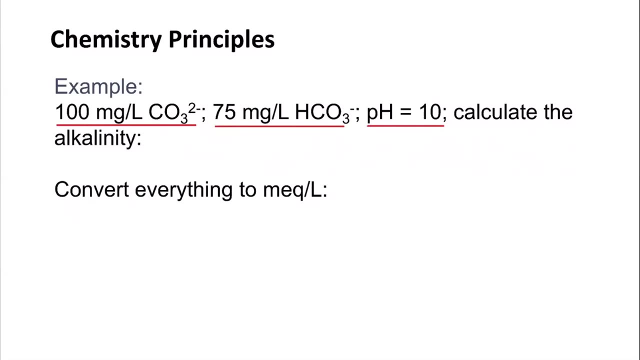 this amount of the carbonate ion. okay, Note that here we are using the mass concentration. okay, So this amount of bicarbonate ion and we know the pH. So what is the alkalinity according to our definition? right? So you can do a quick calculation or at least show the equation to. 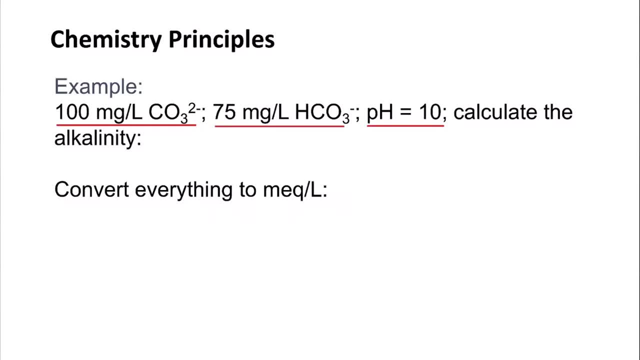 do this calculation. Okay, I'll give you maybe two minutes to look at this question. Okay, let's go ahead and look at this question, Okay, so this is a very simple example of what we can do to calculate the alkalinity of a water sample. 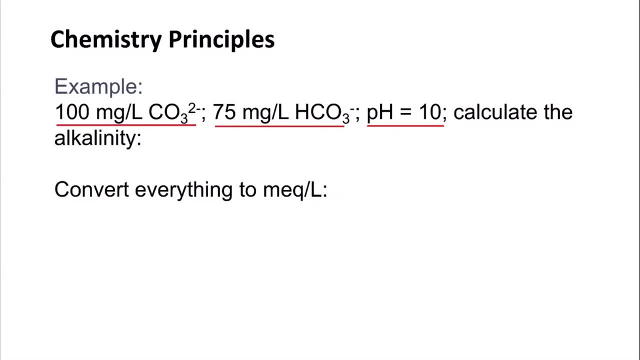 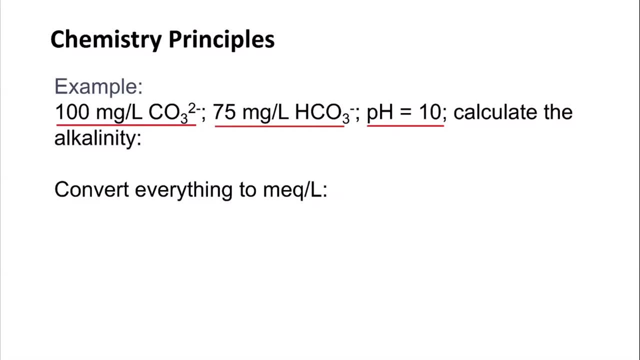 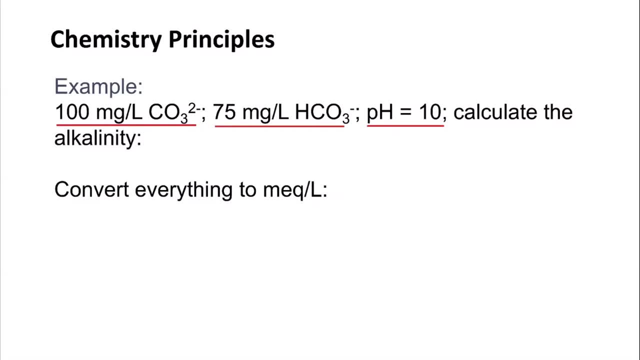 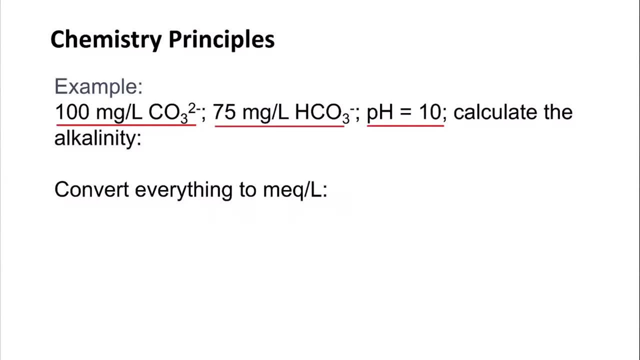 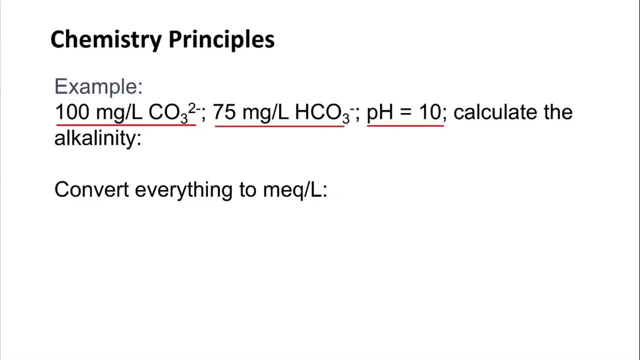 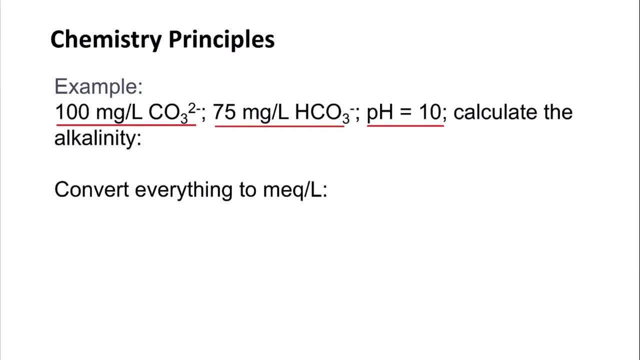 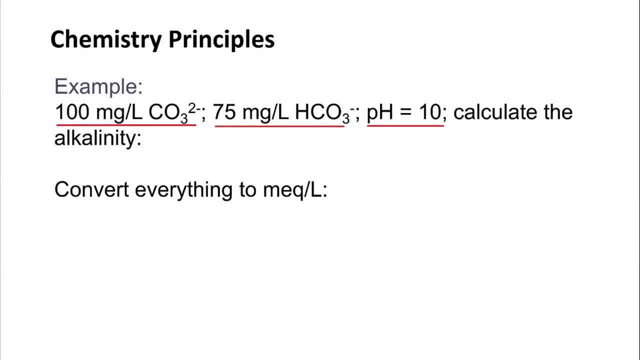 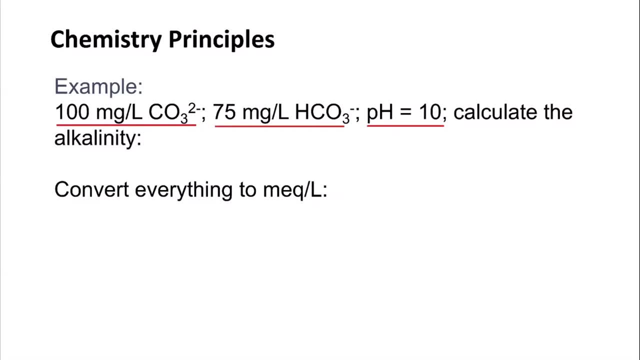 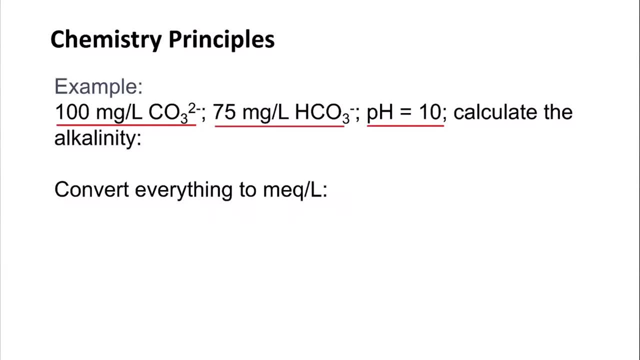 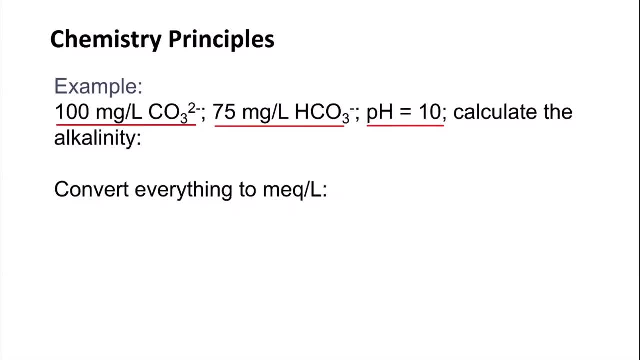 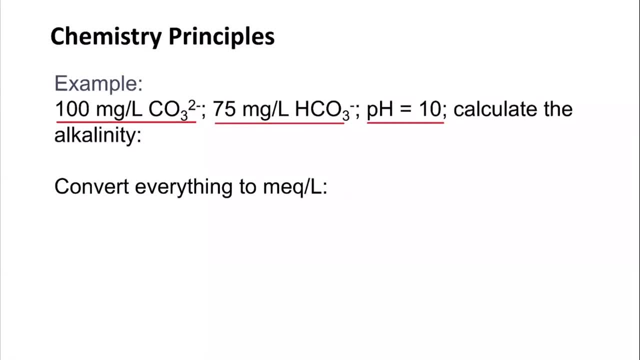 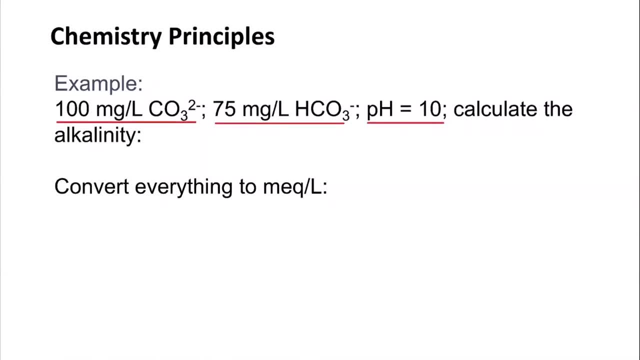 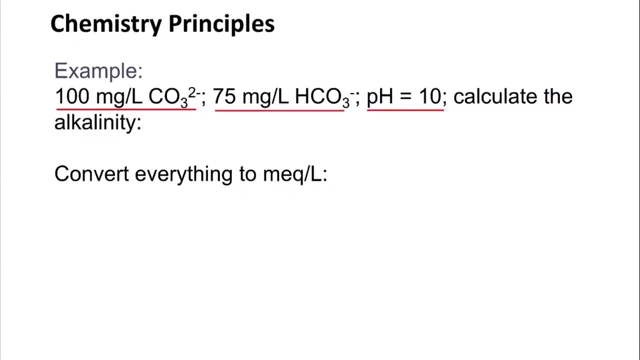 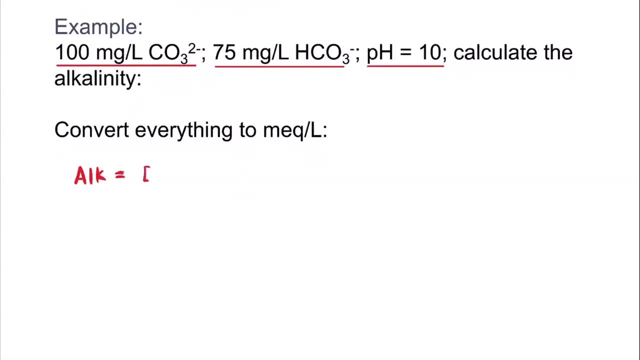 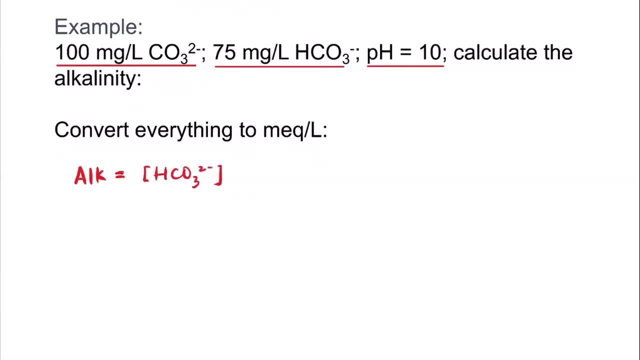 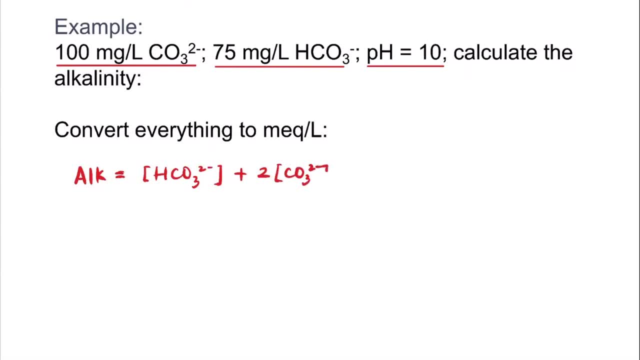 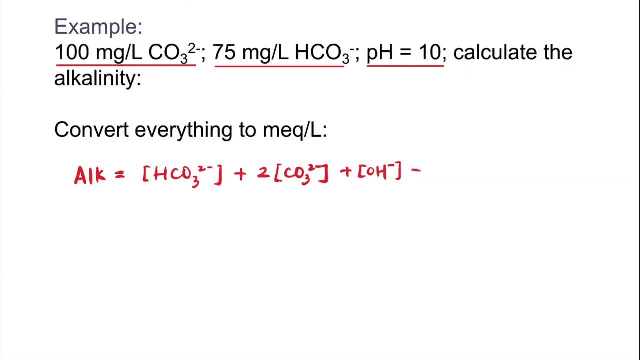 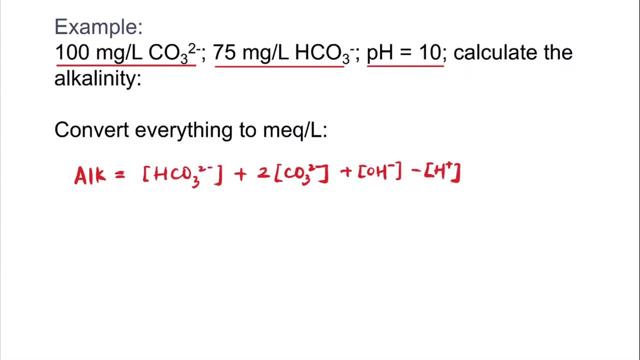 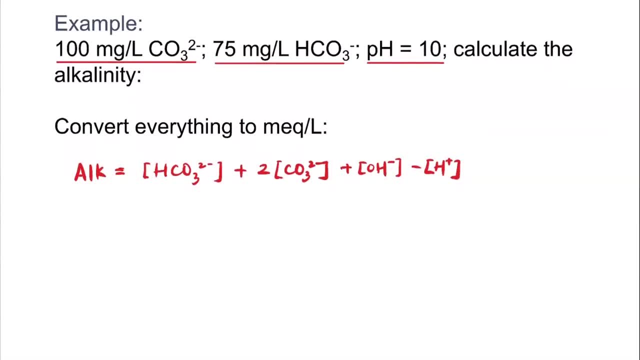 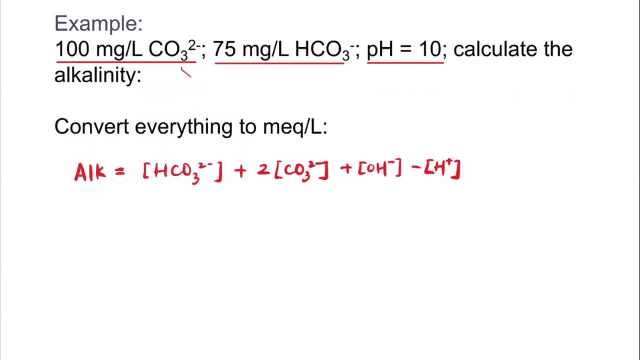 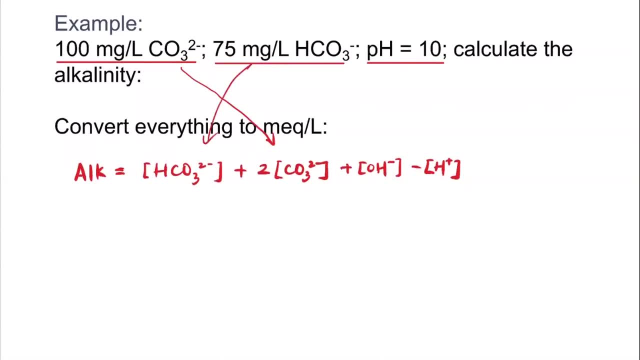 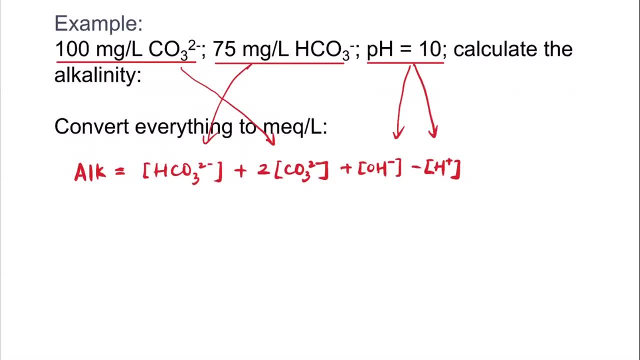 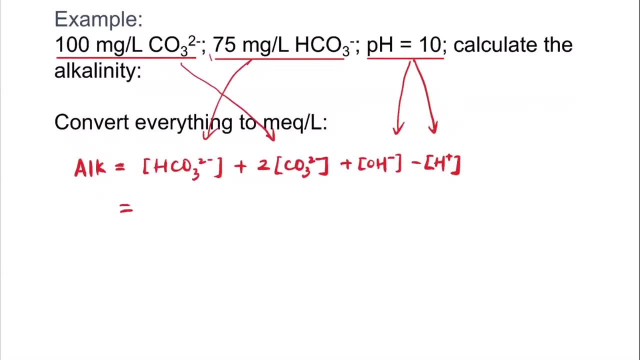 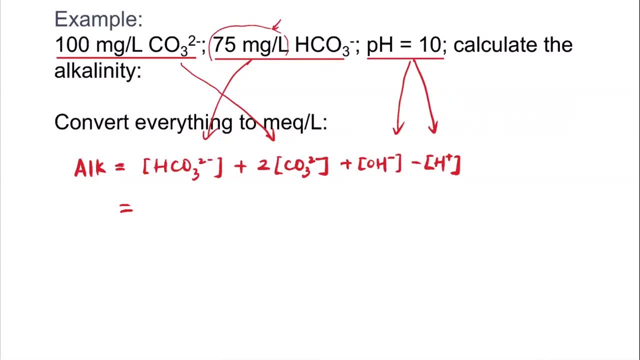 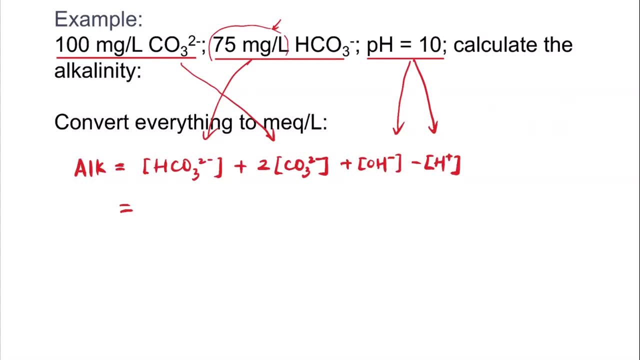 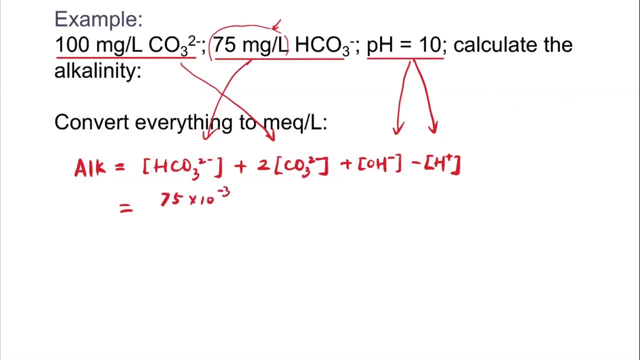 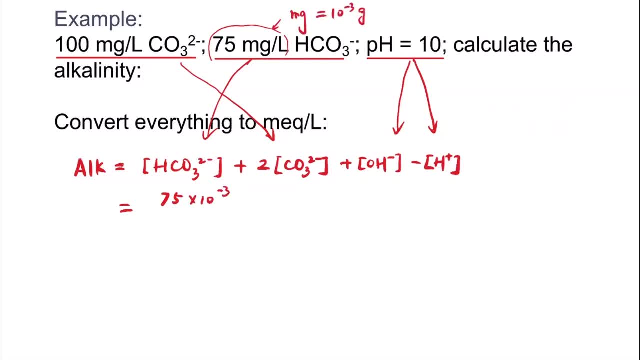 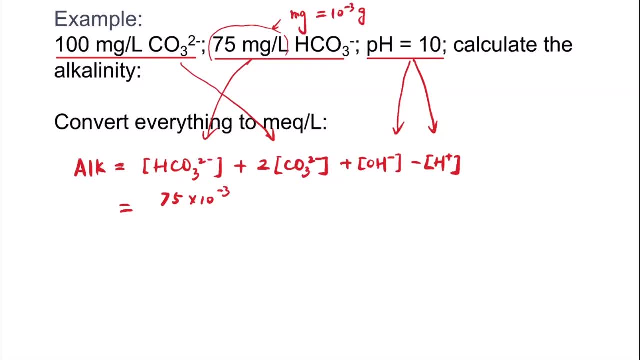 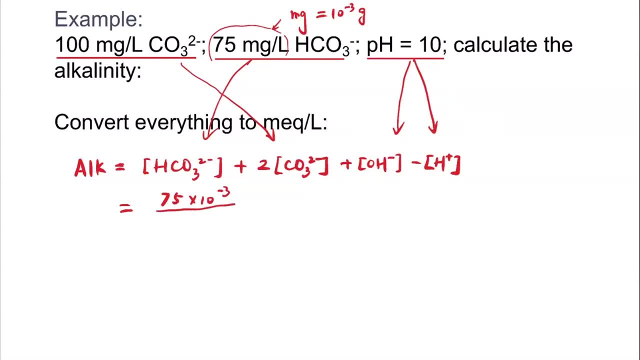 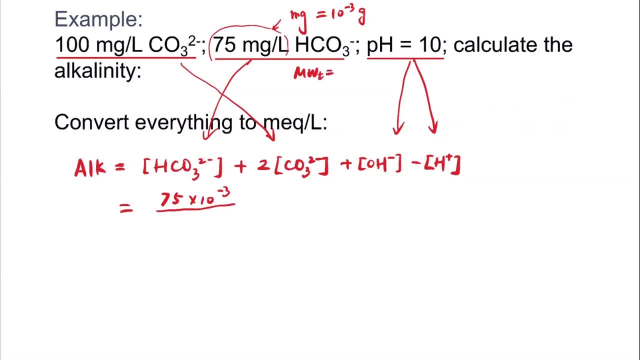 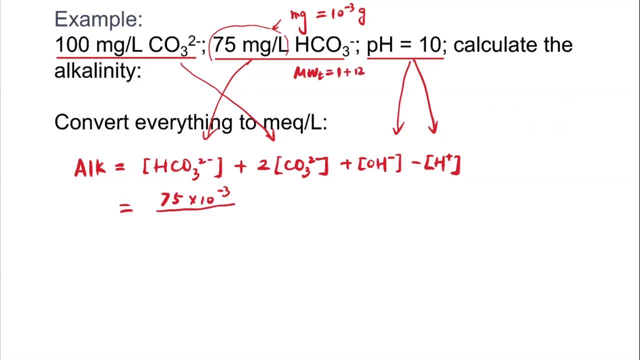 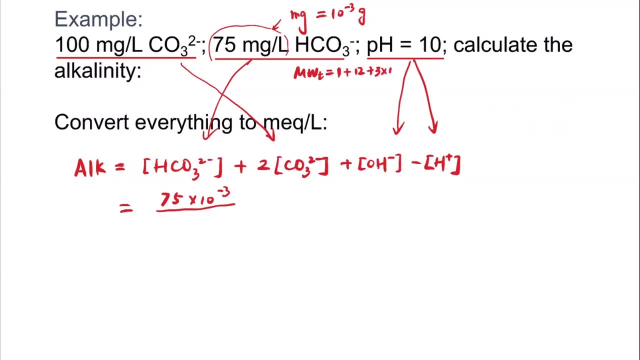 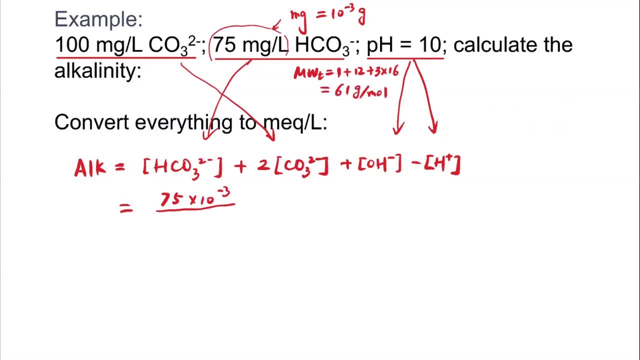 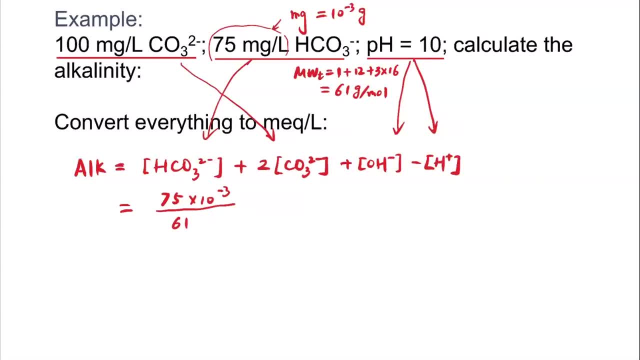 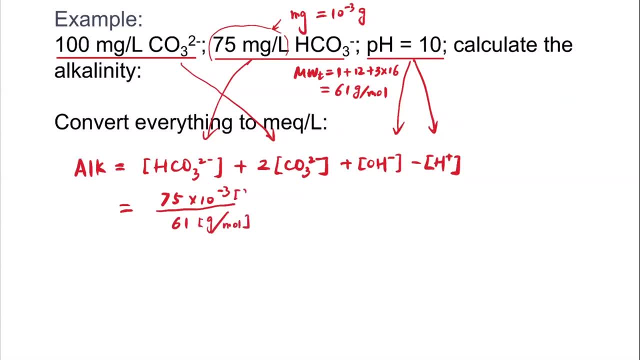 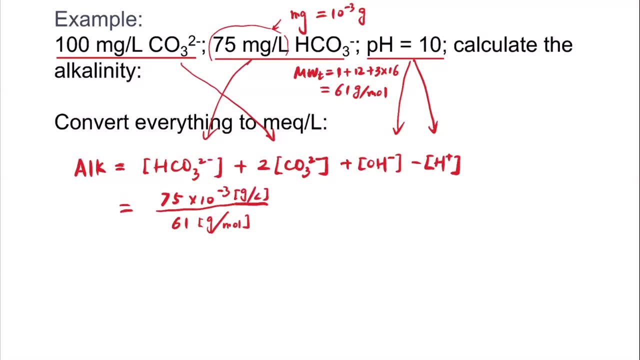 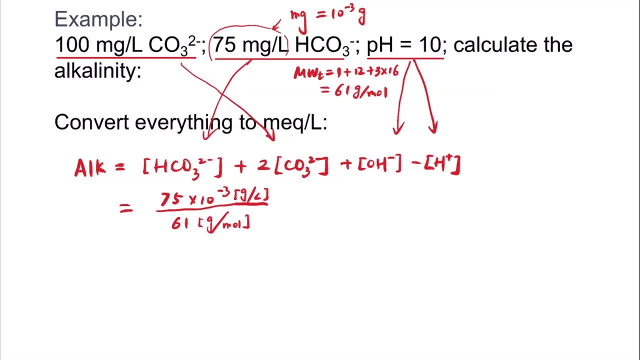 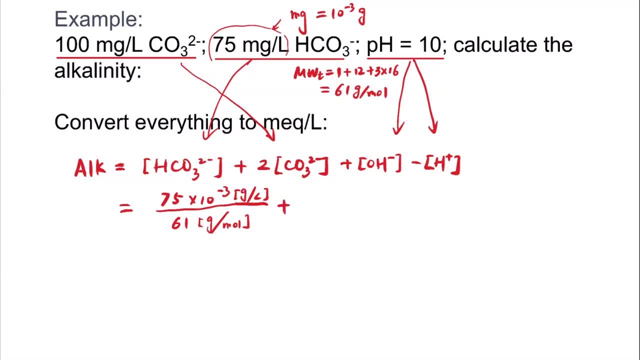 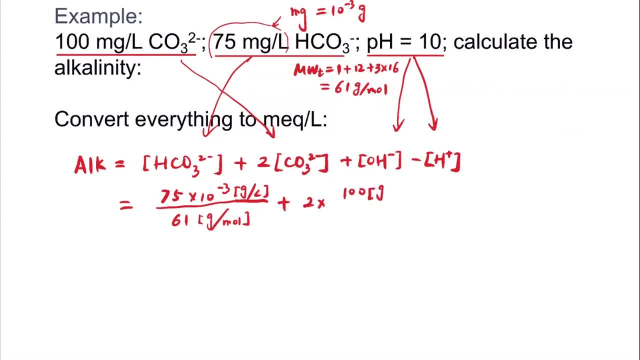 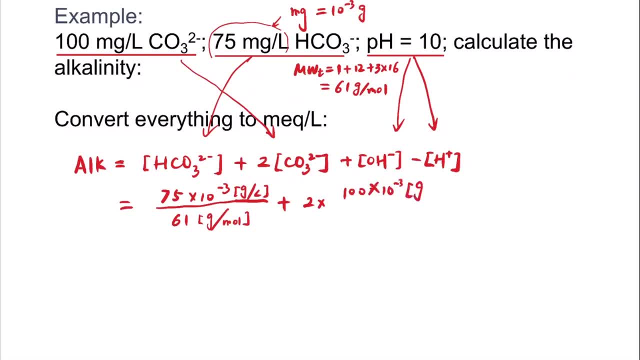 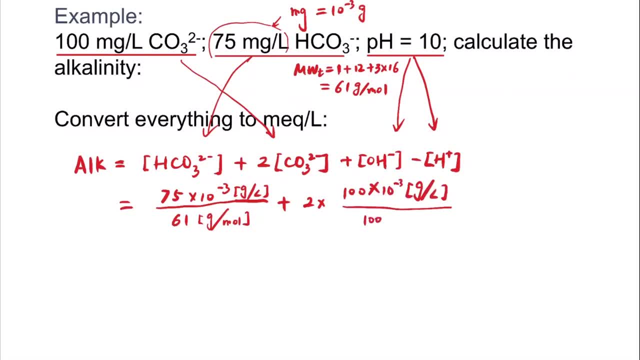 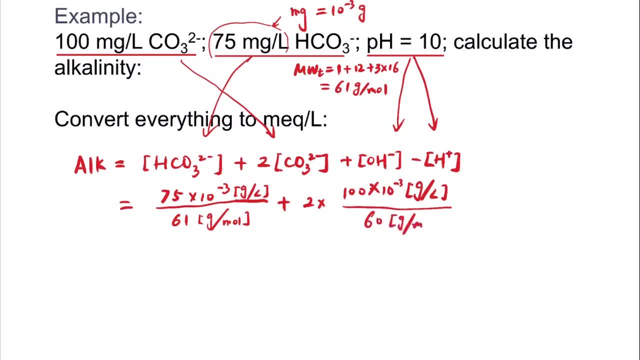 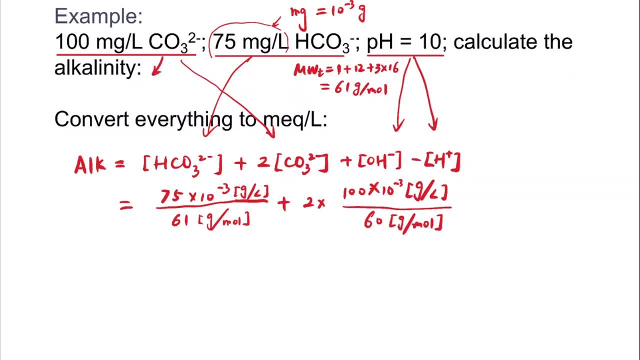 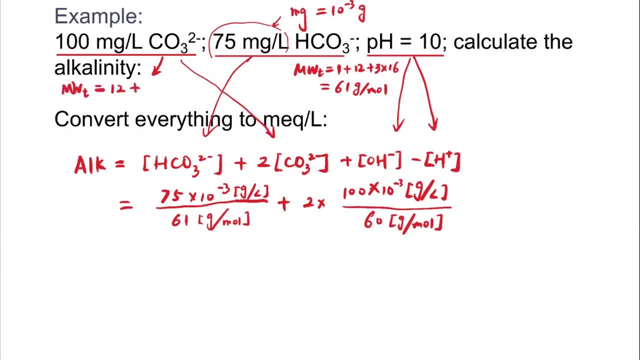 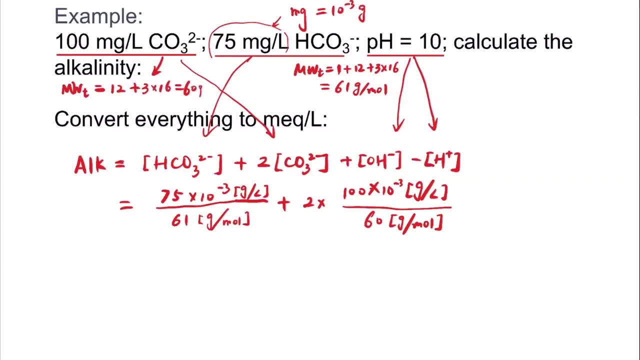 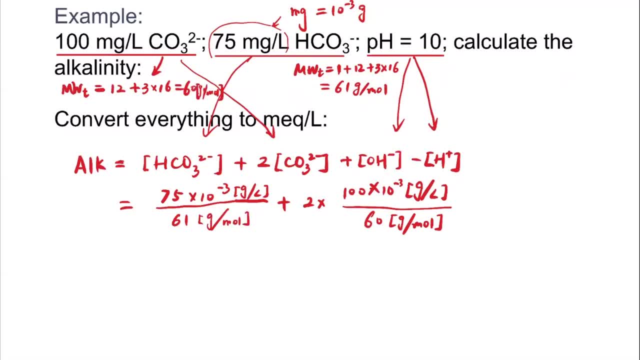 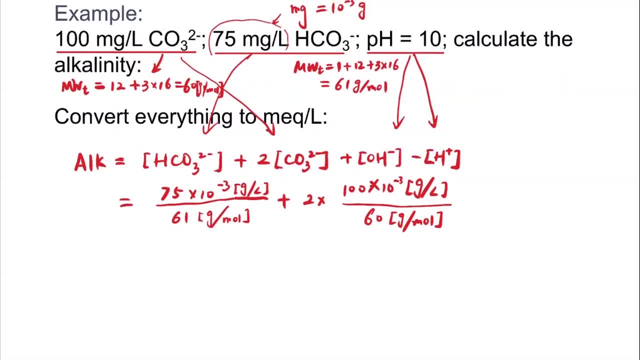 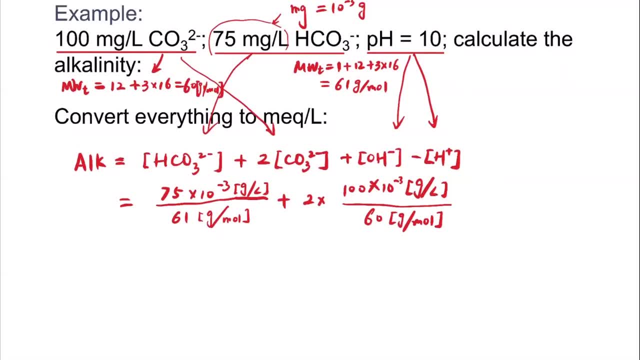 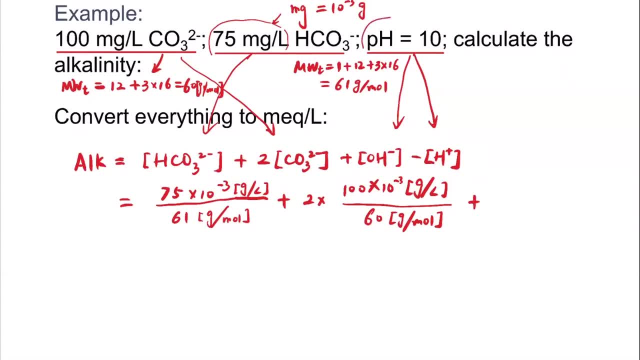 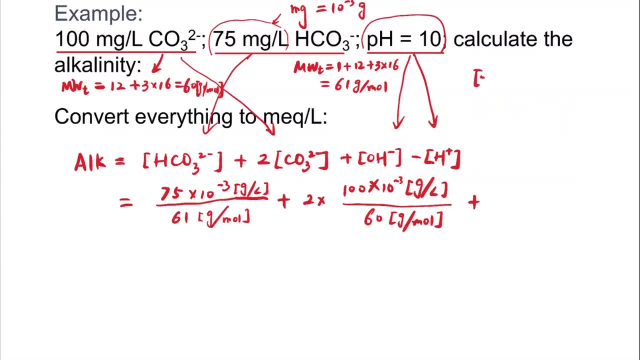 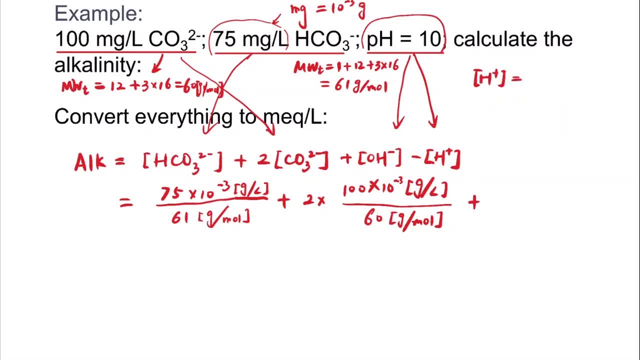 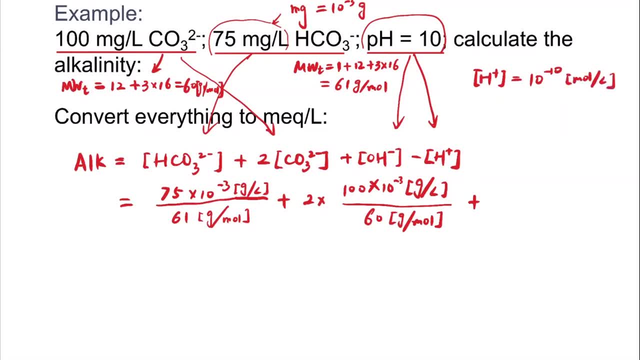 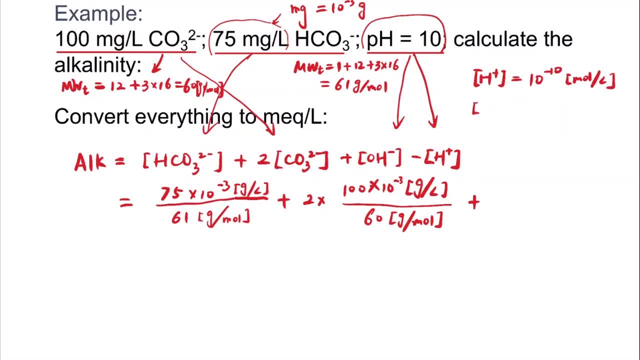 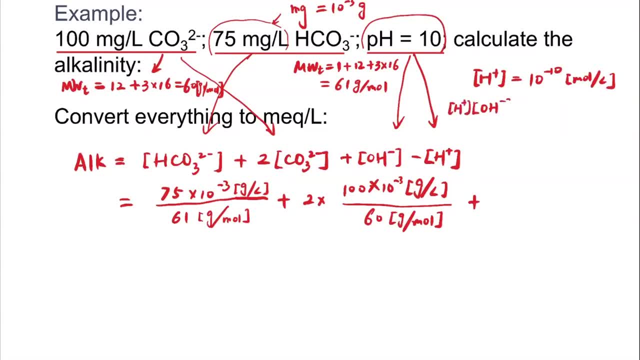 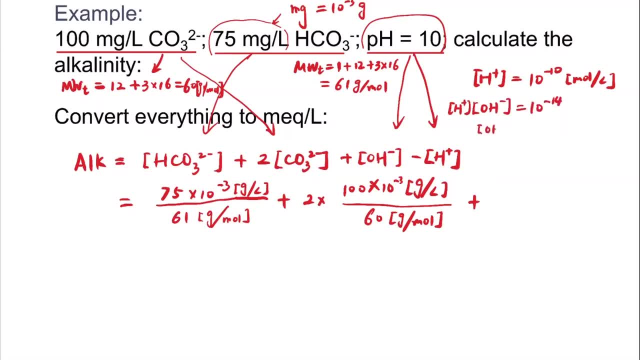 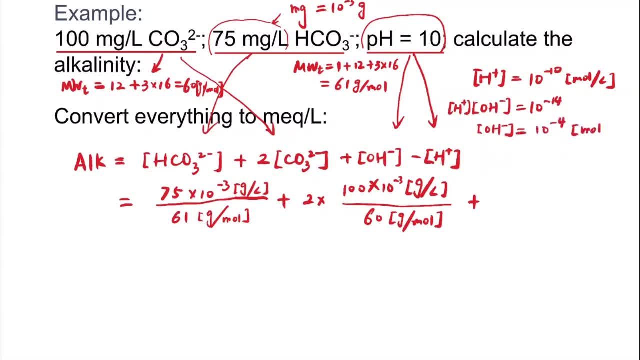 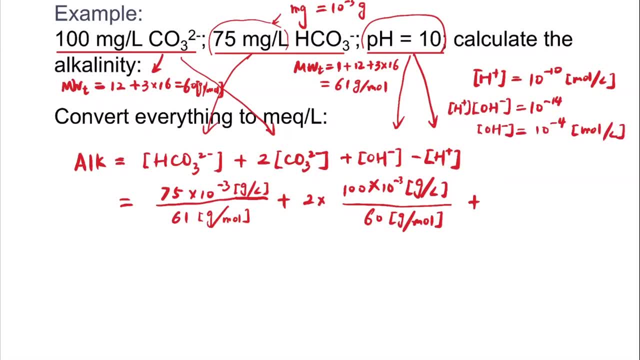 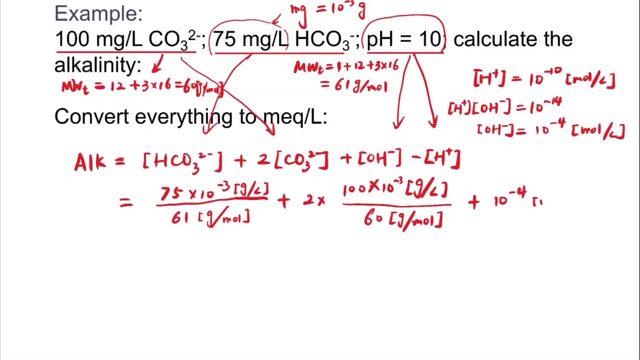 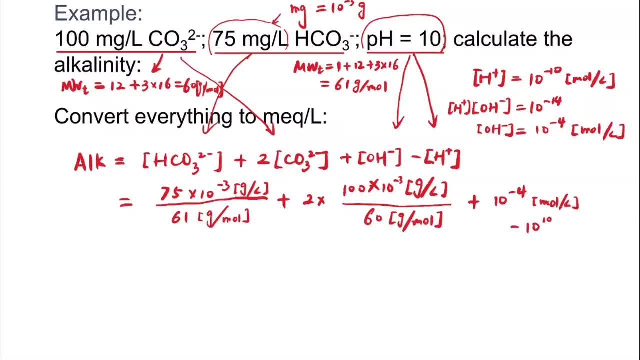 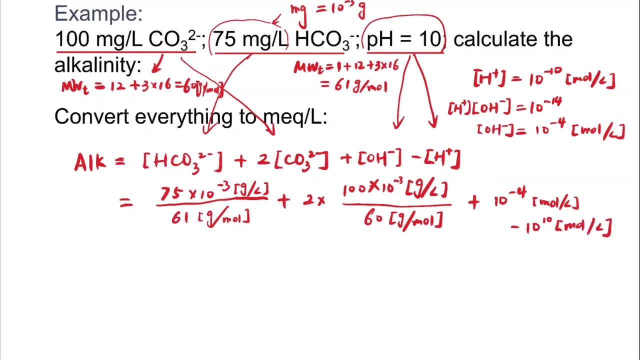 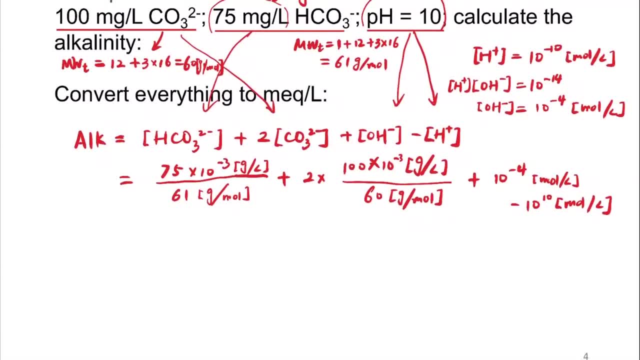 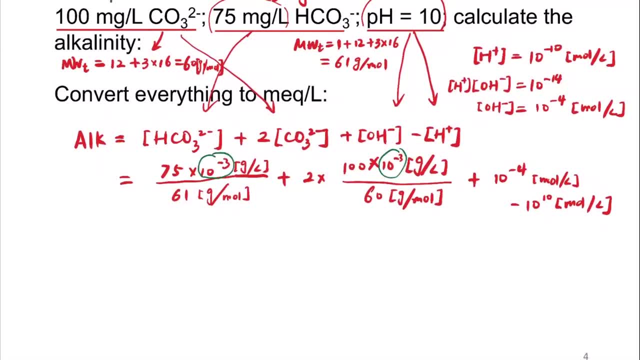 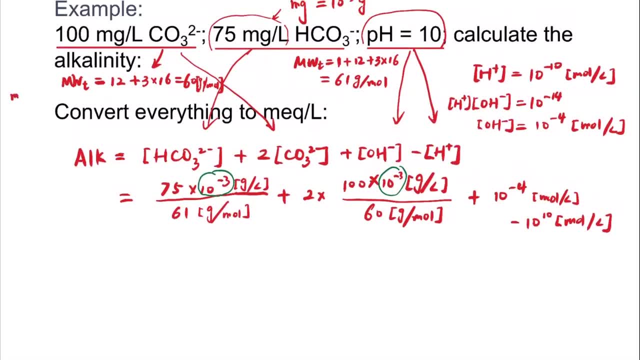 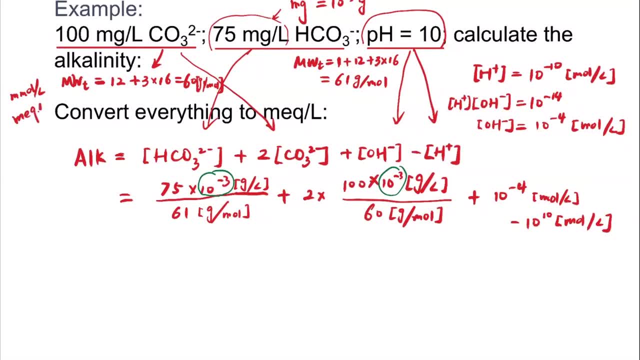 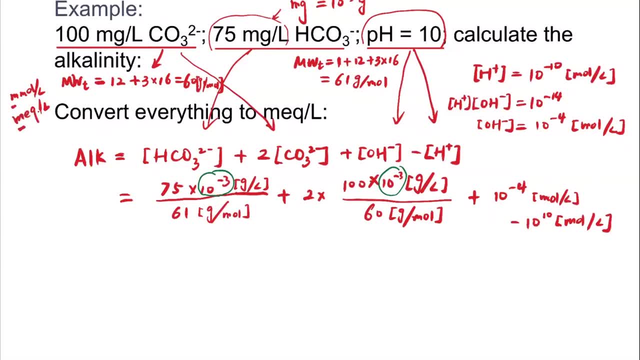 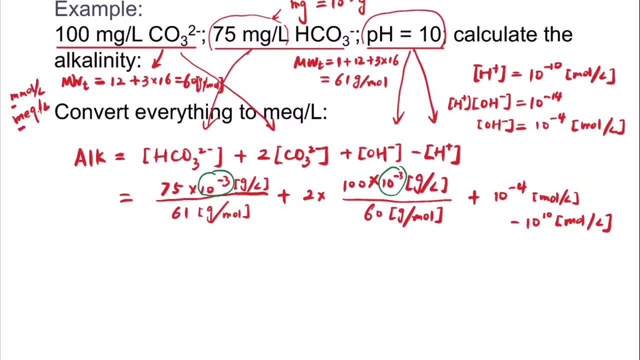 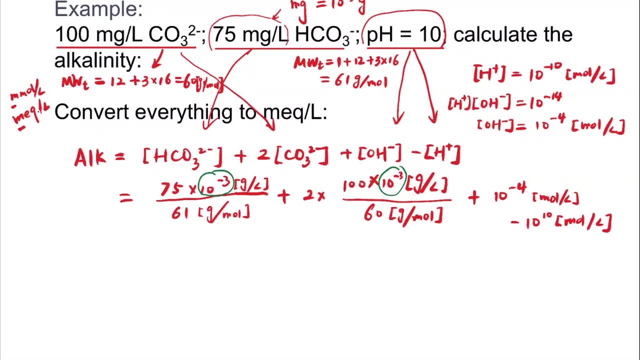 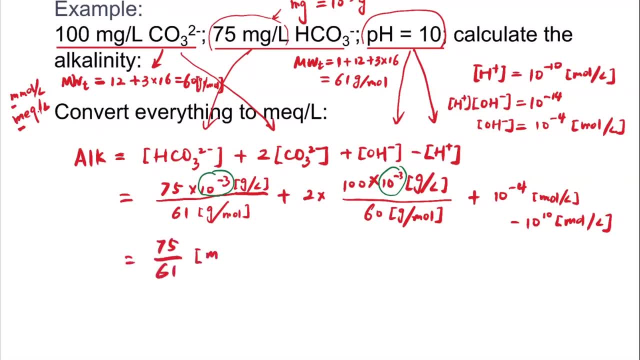 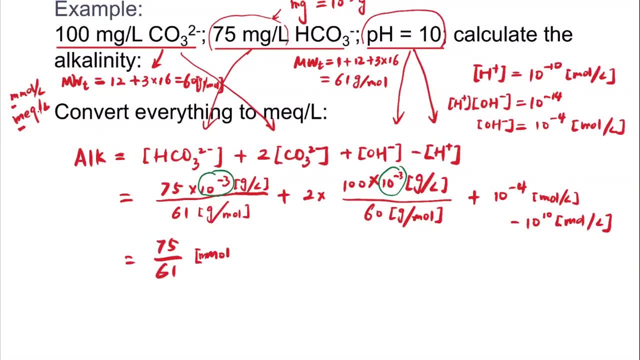 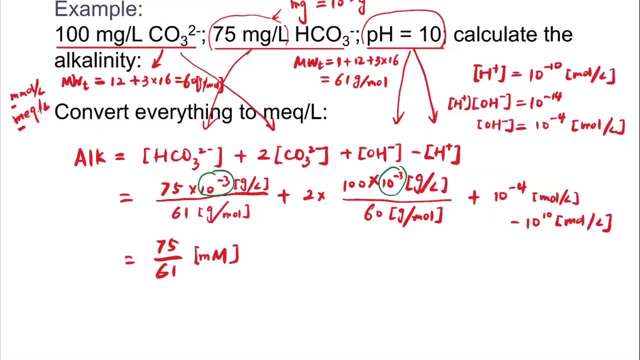 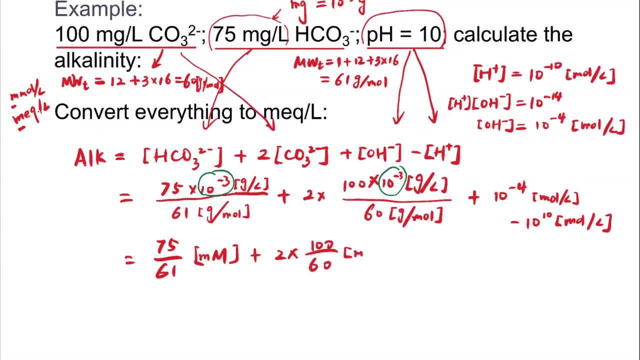 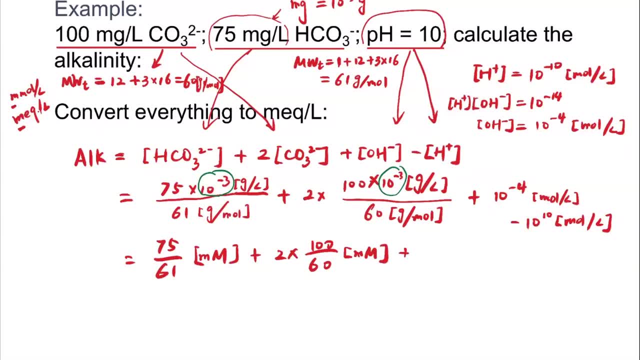 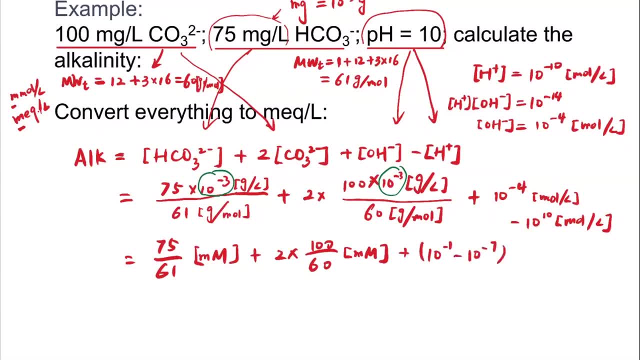 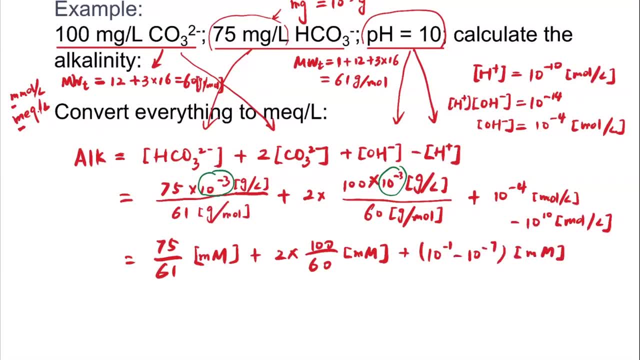 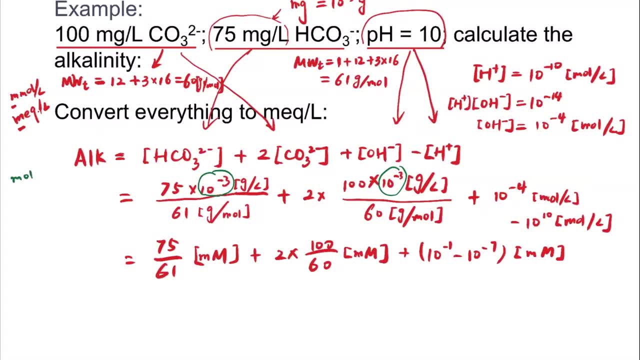 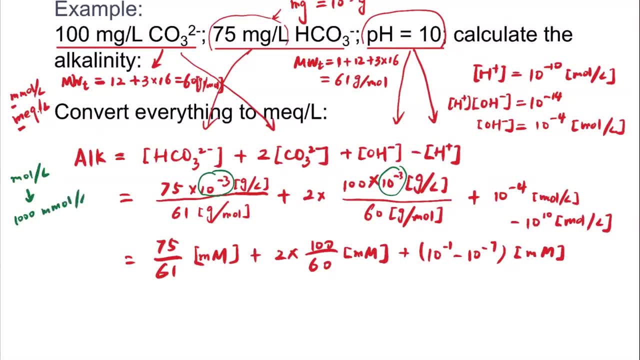 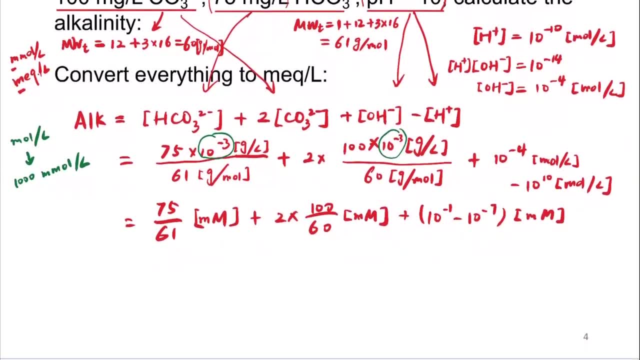 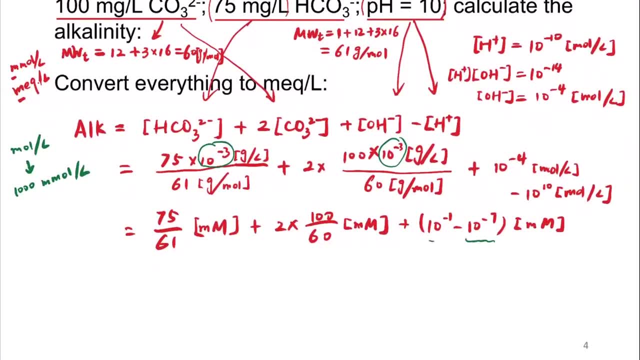 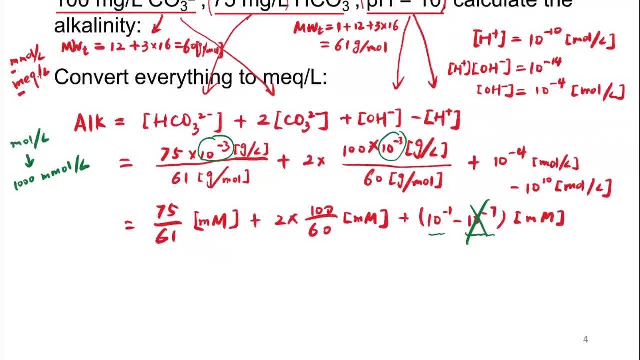 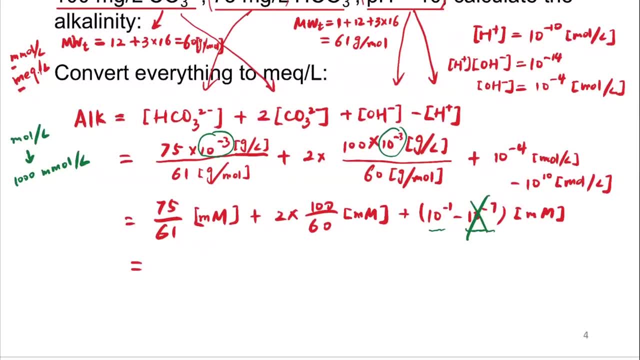 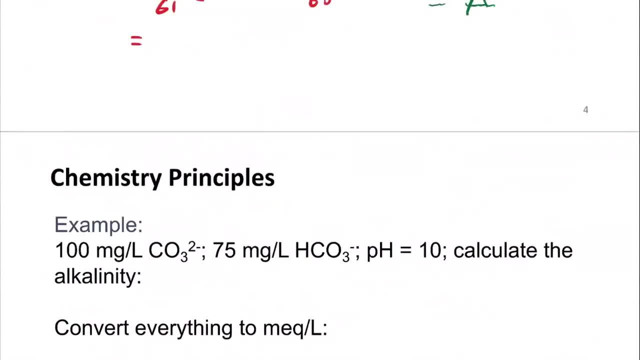 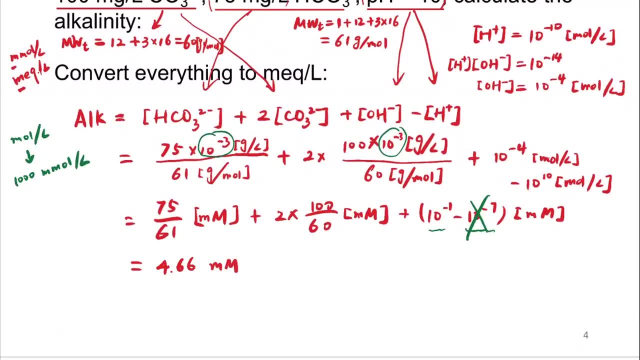 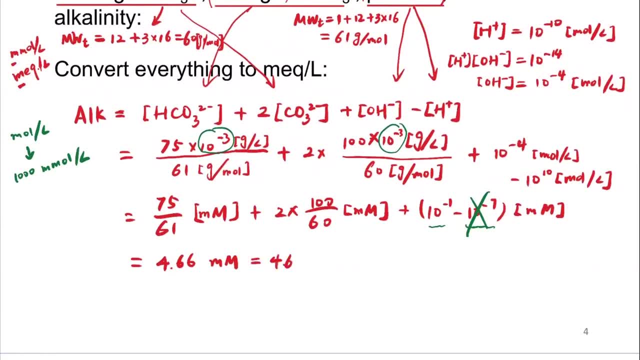 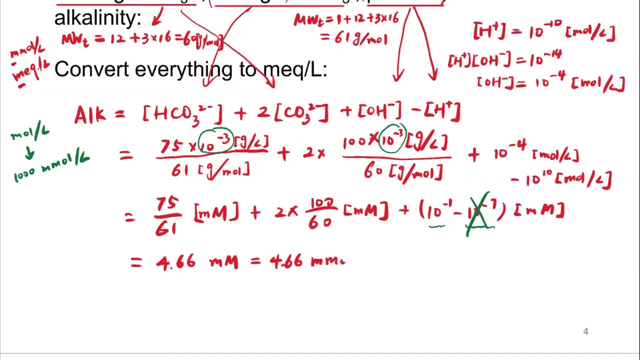 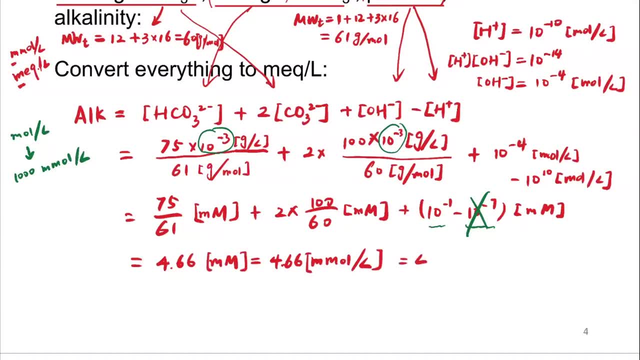 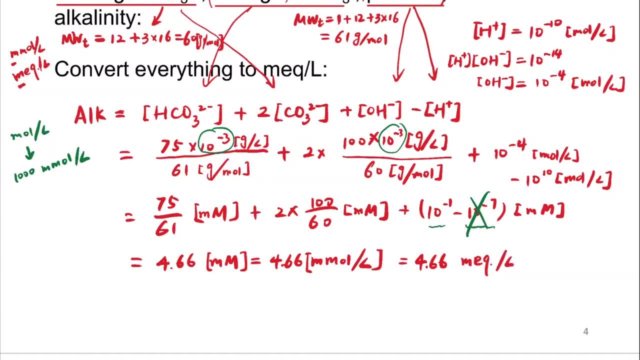 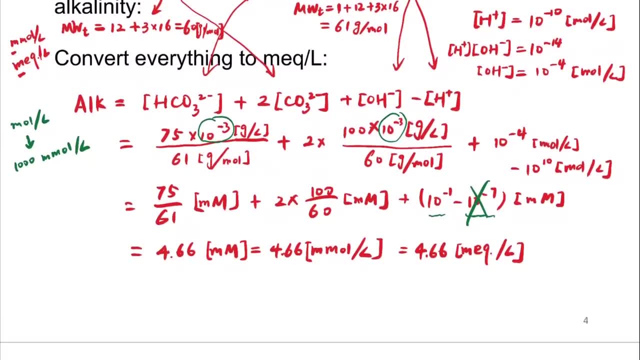 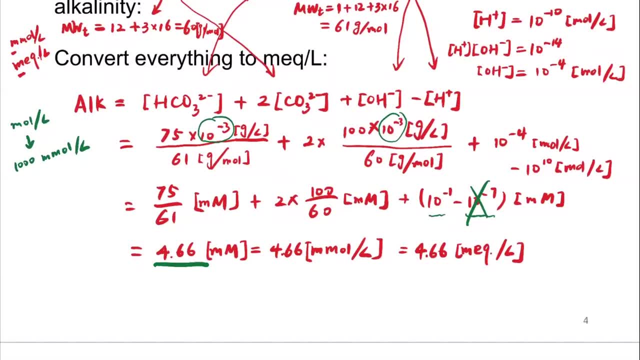 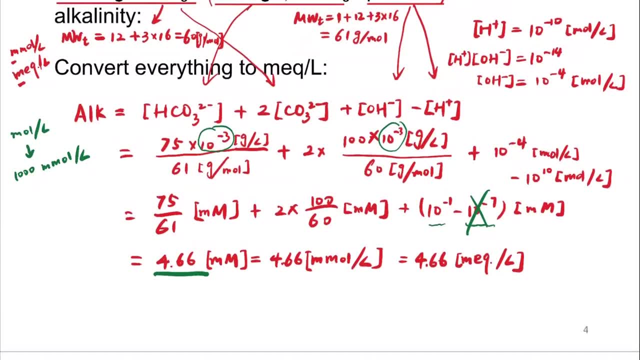 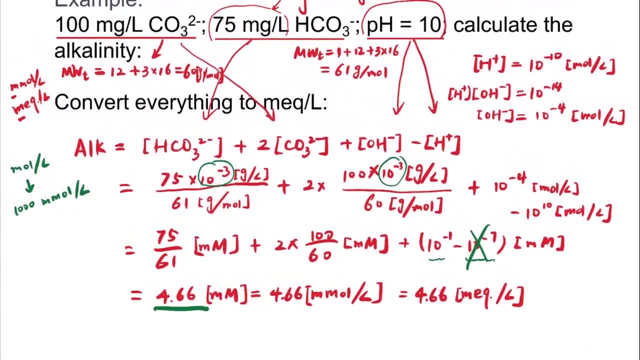 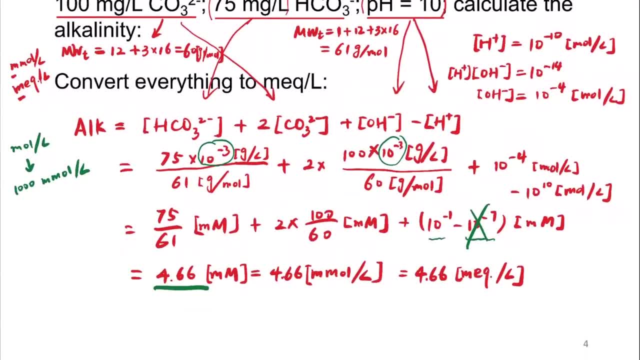 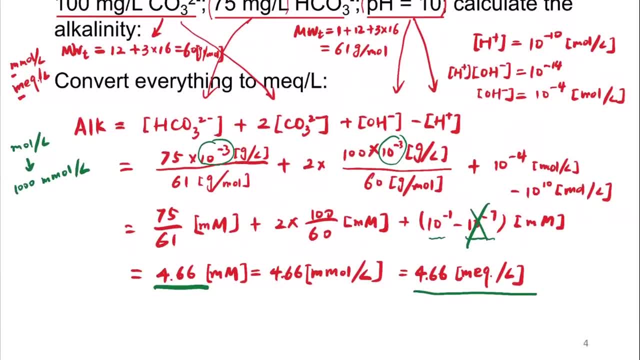 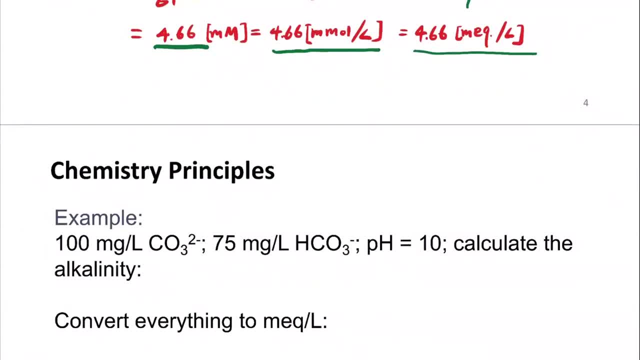 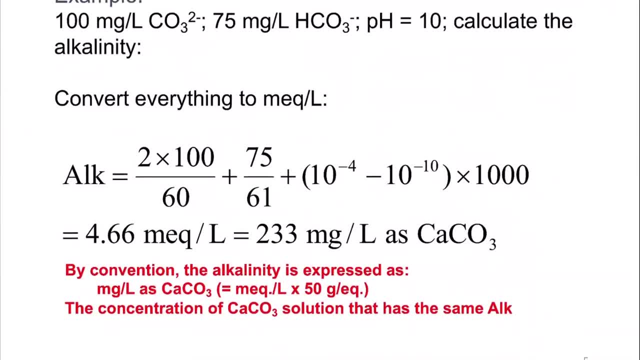 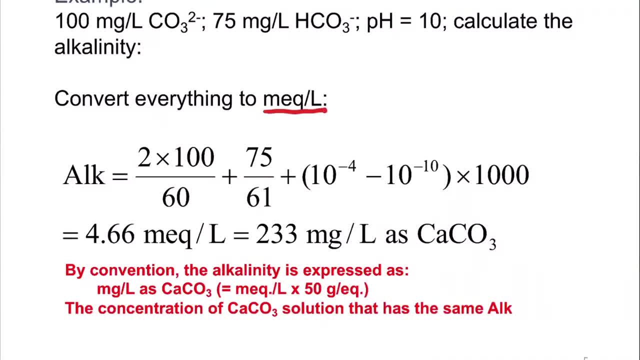 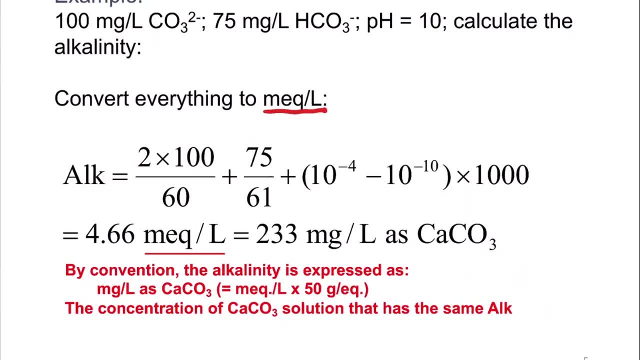 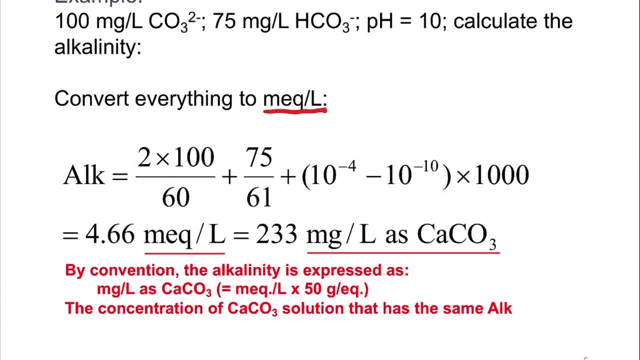 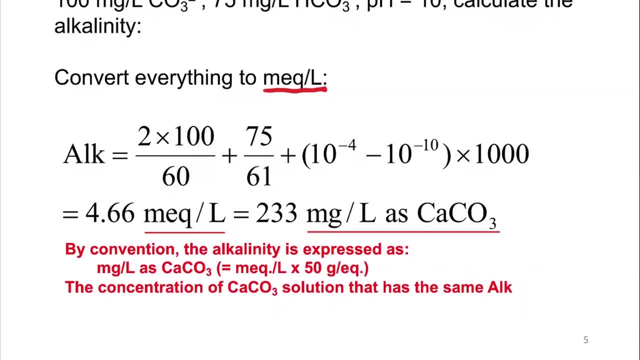 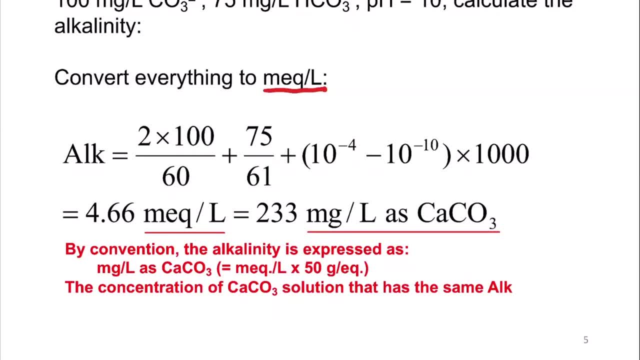 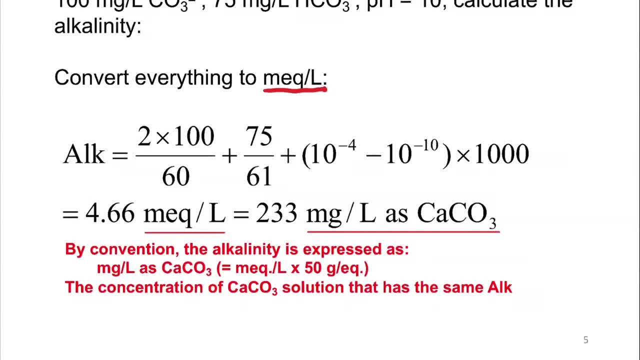 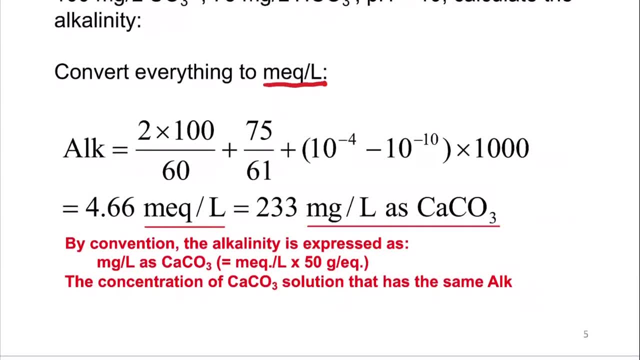 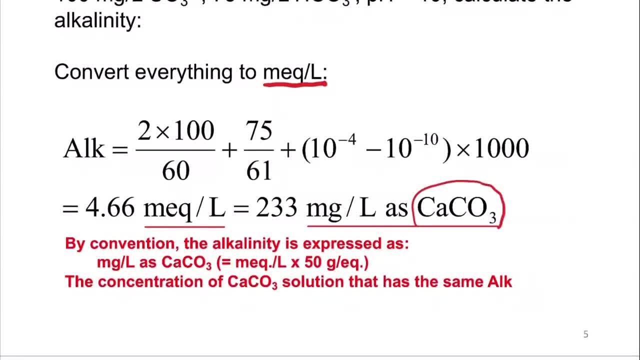 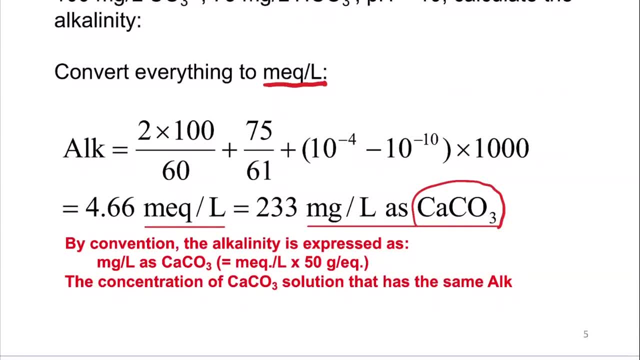 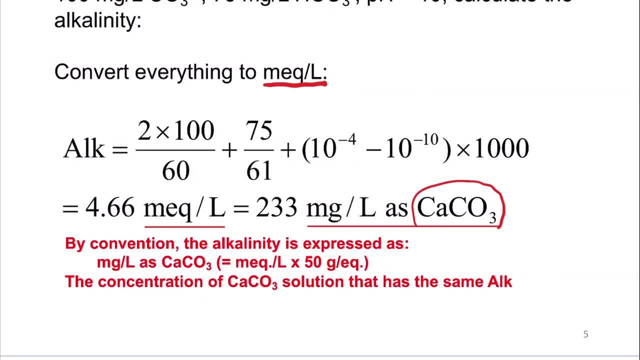 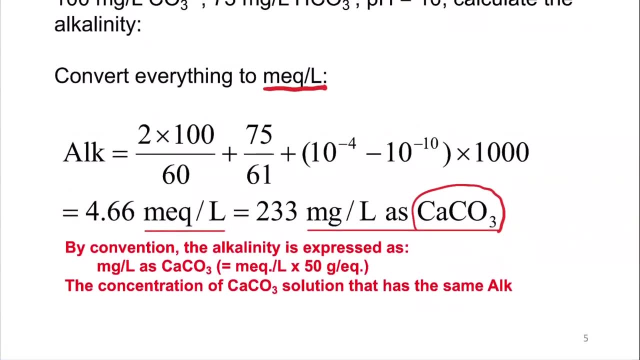 Okay, so this is a very simple example of what we can do to calculate the alkalinity of a water sample. Okay, so this is a very simple example of what we can do to calculate the alkalinity of a water sample of limestone. So for this conversion here, what it means is that we want to find out what is the 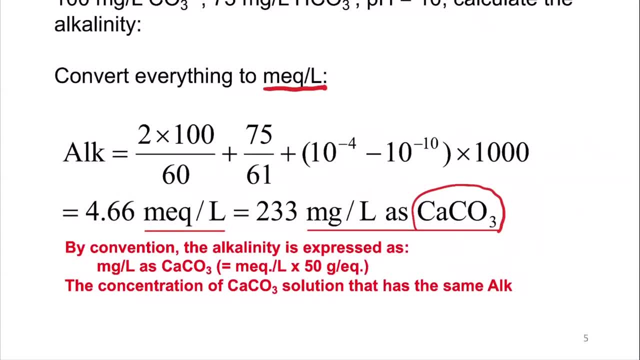 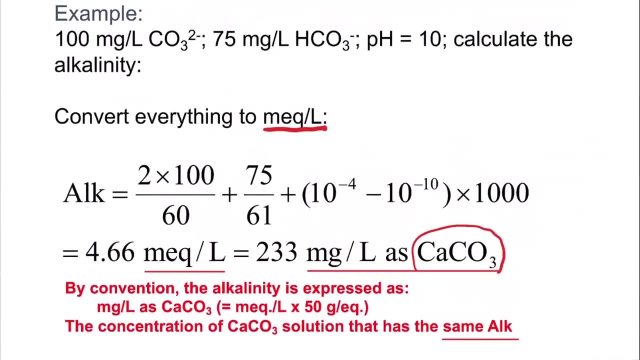 mass concentration of a solution that contains calcium carbonate that has the same alkalinity with the solution that we're trying to look at. So what is the mass concentration of the calcium carbonate that has the same alkalinity? So it turns out that to do this calculation, 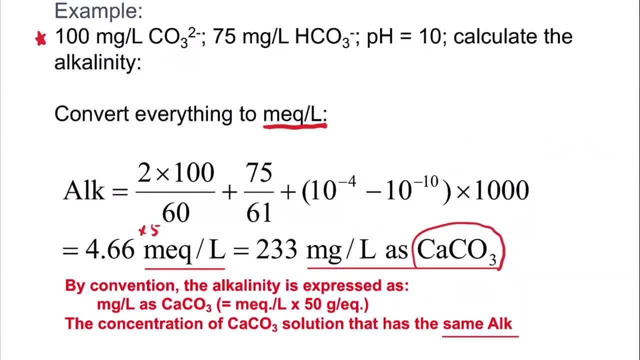 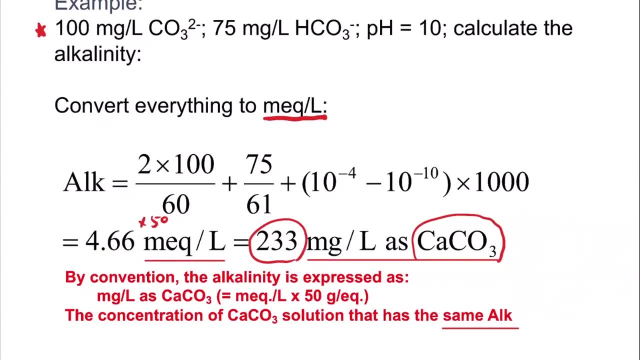 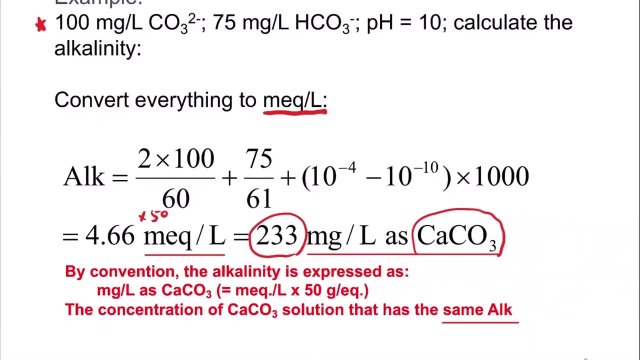 what you need to do is just multiply this value by 50.. So by multiplying this value by 50, you can convert it into: or basically, the result is 233 milligram per liter as calcium carbonate. So this is trying to do an analogy. So for this water sample here, 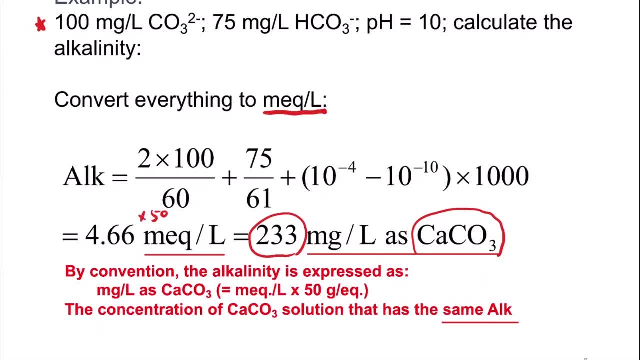 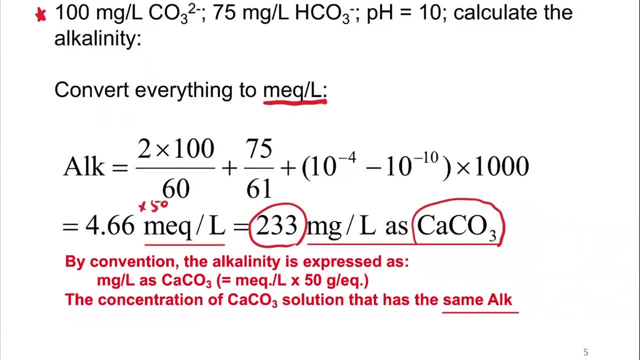 it's alkalinity, It's not the mass concentration of the solution that contains calcium carbonate. The alkalinity is the same as the water sample that contains 233 milligram per liter of calcium carbonate in the water, So they two have the same alkalinity. So then you may wonder how we get this. 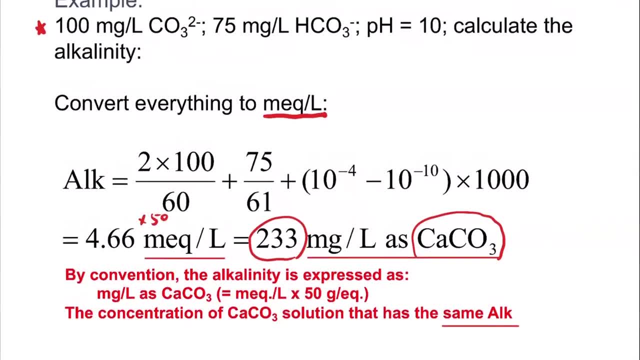 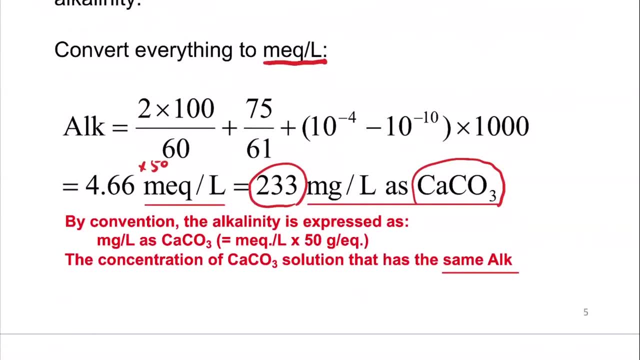 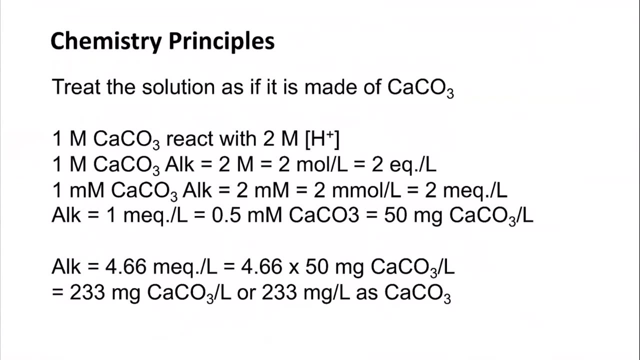 It is quite easy to memorize this. You just multiply it by 50 and then you get what you want. But you can actually try to find out. why do we have this same alkalinity in here? So the method we can use is: let's imagine that we have a solution that contains 1m of calcium carbonate, So 1m. 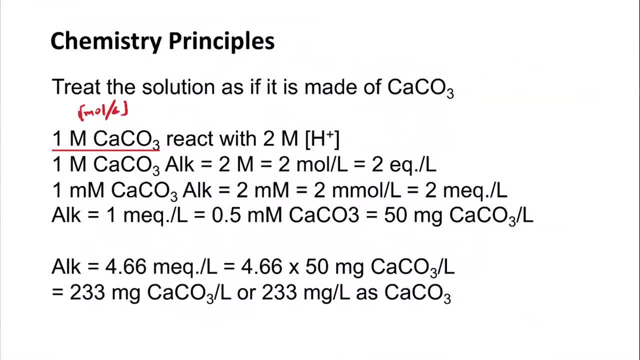 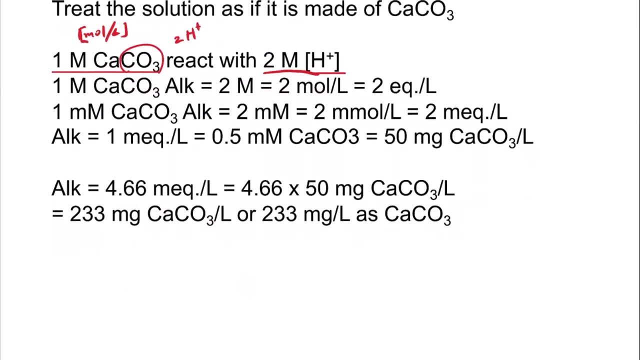 is 1 mole per liter. So for this solution here, we know that when it reacts with the hydrogen ions, it's going to react with 2m of the hydrogen ion, because each carbon ion is going to react with two hydrogen ions. Okay, So because of that, for this solution, if we want to know its alkalinity, then it's just. 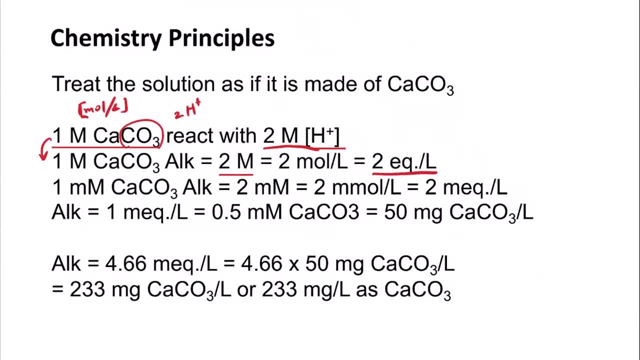 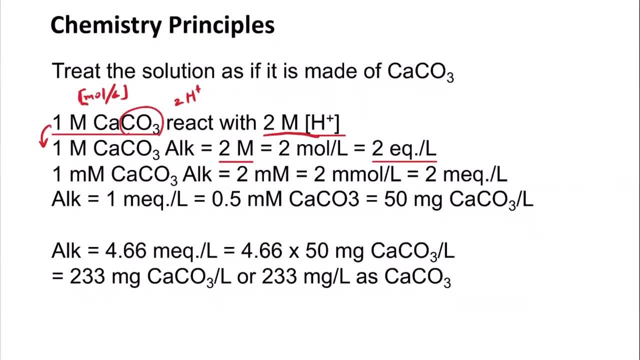 going to be 2m, or two equivalent per liter. Okay. So similarly, let's convert it into milli-m, So 1 milli-m of the calcium carbonate is going to have the alkalinity of two milli-equivalent per liter. Okay, So what this also means is that if we just rewrite it in this way, okay, so then. 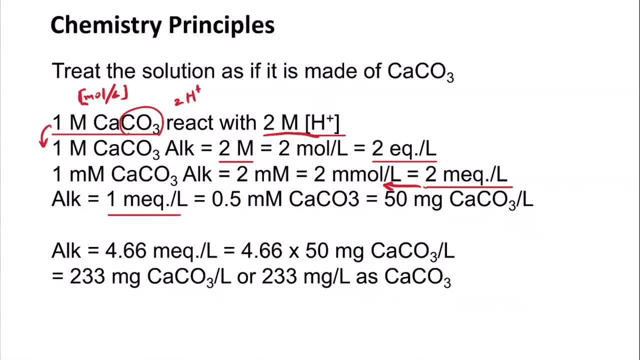 1 milli-equivalent per liter means 0.5 milli-m of the calcium carbonate. Okay, So 0.5 milli-m just means 0.5 milli-mole, or 0.5 multiplied by 10 to the negative 3. 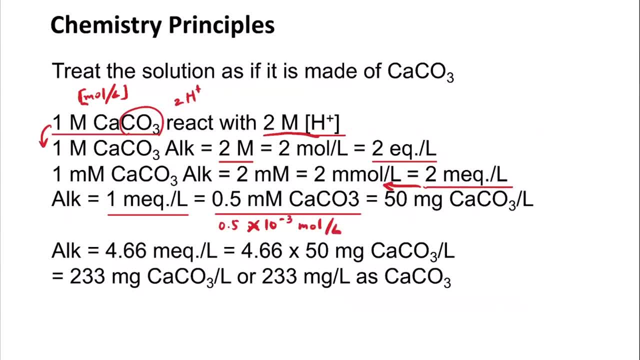 mole per liter. Okay. So what is the mass concentration of calcium carbonate if we have this solution? Okay, So we just multiply this by 100 gram per mole. Okay, Because the molecular weight of calcium carbonate is 100. Right, So what you get is basically 0.05 gram per liter. Okay, So 0.5 gram per liter is equal to. 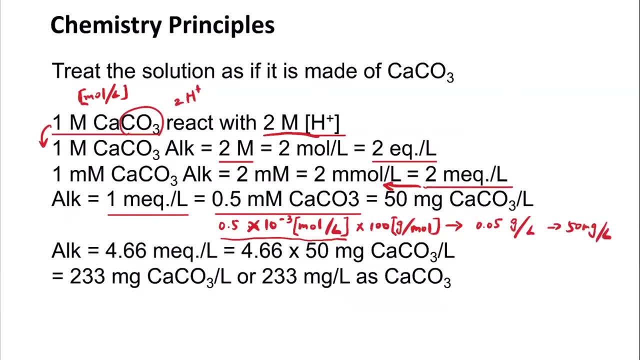 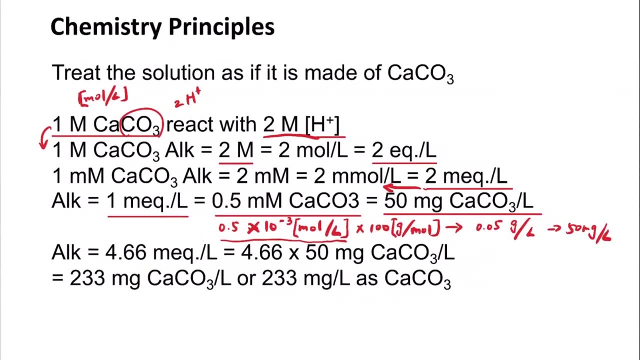 50 milligram per liter, Right? So basically, 1 milli-equivalent per liter means 50 milligram of calcium carbonate In terms of the alkalinity. Okay, So now, basically, by knowing this conversion, we know that 1 milli-equivalent is equal to 50.. Then, for this problem, we have 4.66.. Right. 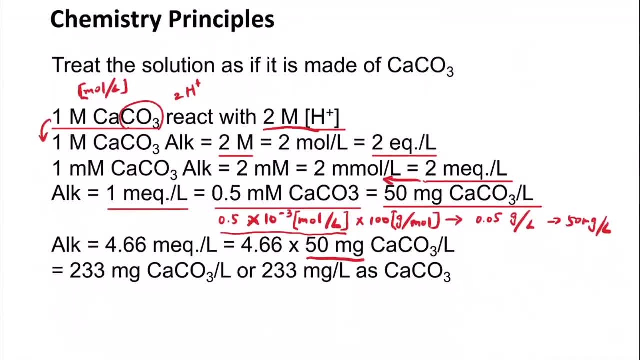 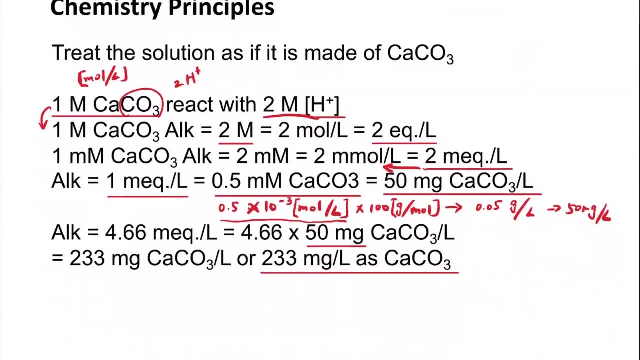 So we just multiply this 4.66 by 50 milligram per liter, And that is going to be the alkalinity that's shown as calcium carbonate. Okay, So this is where this 50 is coming from. How do we convert the alkalinity in terms of the calcium carbonate? Okay, 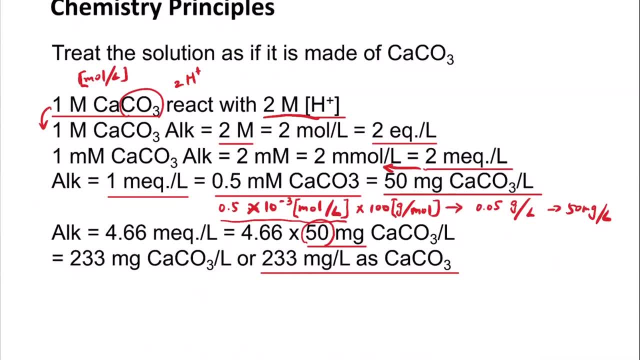 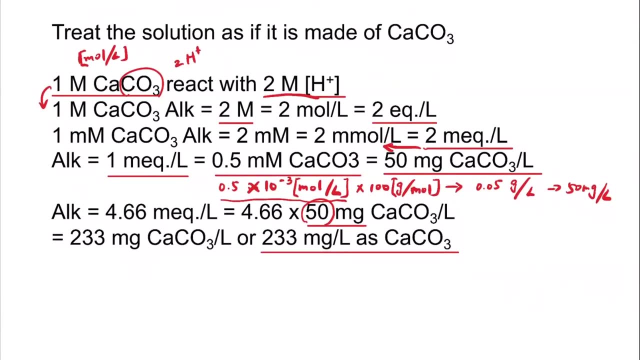 So I know that there are quite many conversions when you solve this problem, But let me know if you have any questions. You also have two homework problems this time to do some similar practice. Okay, So this time I think in the textbook what they also refer to this method as the exact. 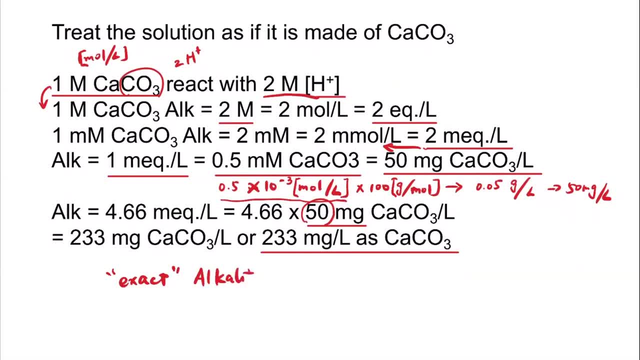 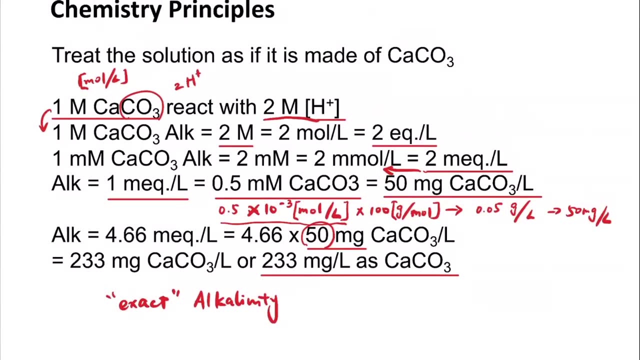 alkalinity, And so I'm going to start with this first one. So let's see, Oh, okay, So let's put it like this: So we have this here, this is the approximate alkalinity. Okay, So, compared to that, you also have the approximate alkalinity. So what? the approximate? 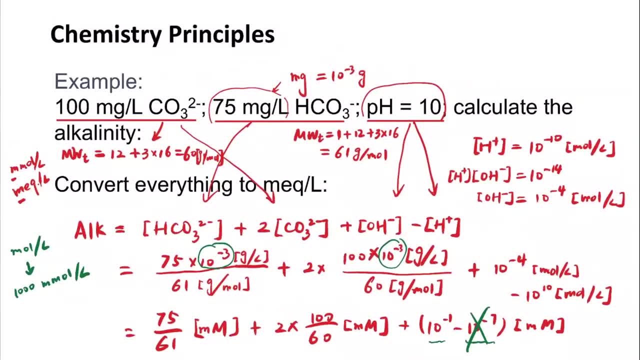 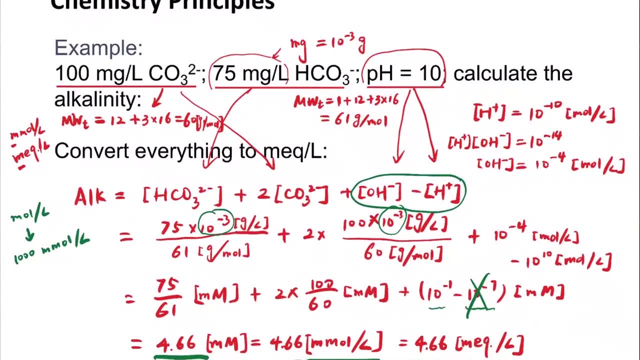 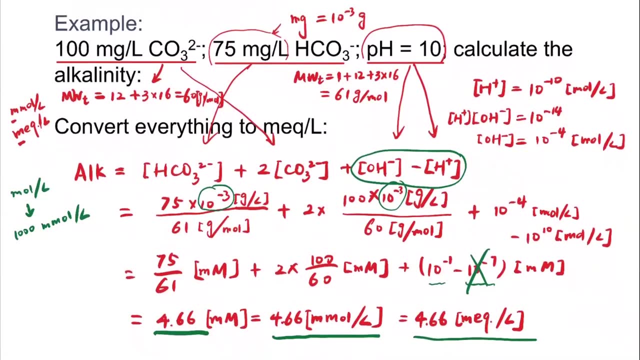 alkalinity means is the calculation. the calculation doesn't, okay. so if the calculation only content considers the bicarbonate and carbonate, then that's approximate alkalinity or rough alkalinity. but when you consider the oh and hydrogen ions, then they are exact alkalinity. okay. so in the homework problem you're going to solve this exact. 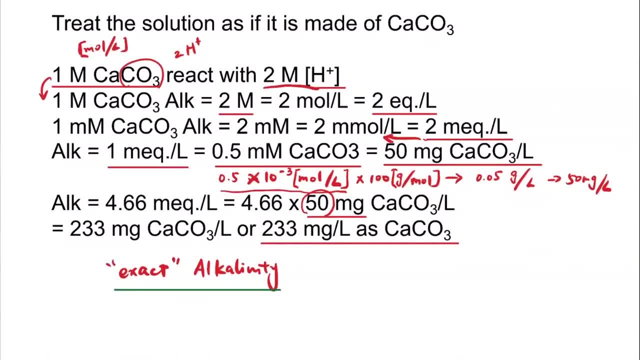 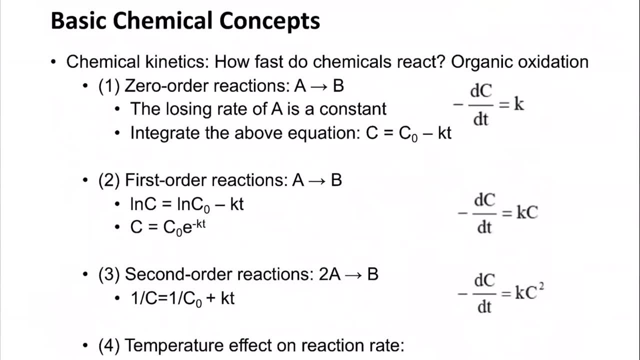 alkalinity there. all right, so this is about the alkalinity and hope, i hope that you're getting a little bit more clear on this concept, okay, so finally, is the reaction, or the chemical kinetics. so we talked to quite a lot about the chemical equilibrium, so this is where all the ions is. 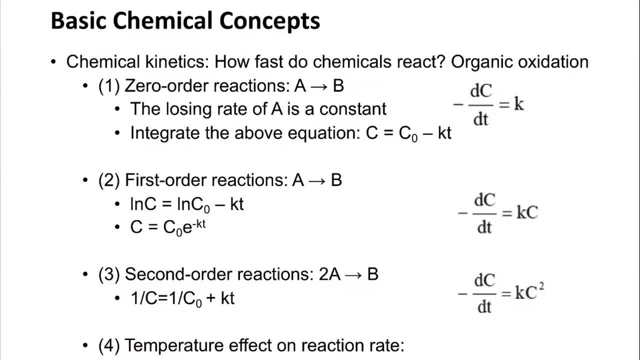 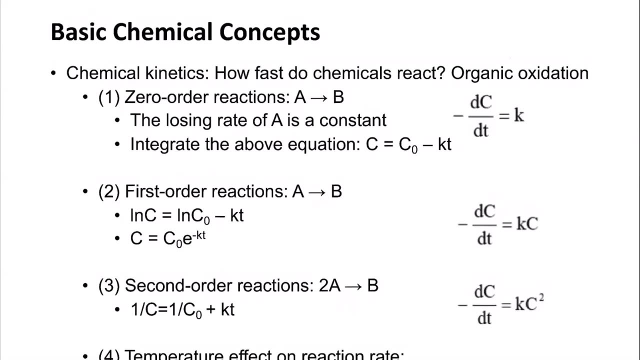 coming out right. so we have the bicarbonate ion, carbon ion, and then they're following the equivalent, equivalent constant. right, you can calculate concentration of the ions, but what the chemical equilibrium describes is the final state. okay, so let's say you have a mixture of ions in a bottle and then 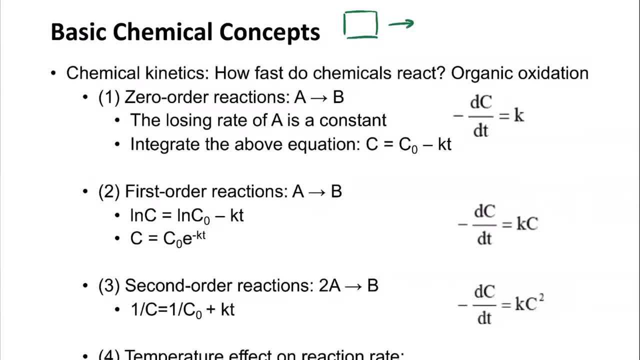 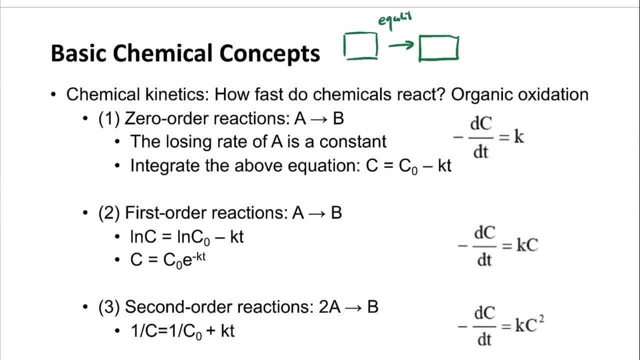 after you place it for some time, it's going to reach to its final state. so that's determined by the equilibrium. but we didn't specify how long it takes for it to reach the final state. it can be one second, it can be one year, it can be thousands of years or like the entire time. 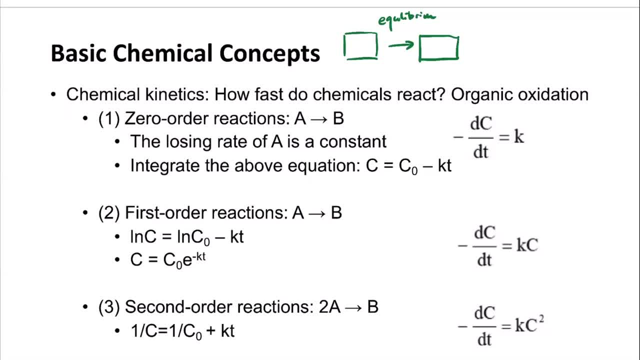 of the universe. so our final state is the final state of the atom. universe is also: it's always not in the equilibrium right because it's always changing. it's not as it's steady, or the final state yet okay, but how do we determine how fast it reached? 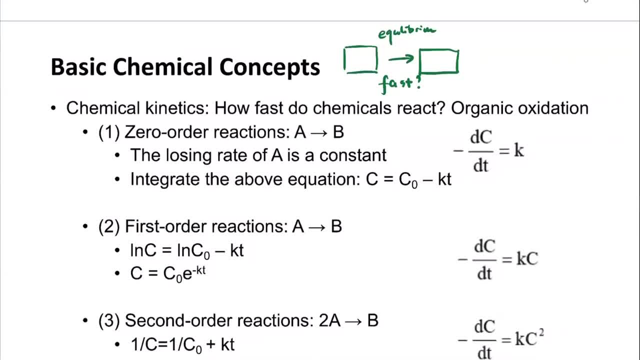 to the equilibrium. okay, so that's going to be the chemical kinetics. so, basically, this chemical kinetics describes, as i said, describes what is the time is needed to reach to the final state. okay, so this is very important for, i would say, the environmental engineering for water treatment or wastewater treatment. that's because if a reaction is happening so slow, let's consider 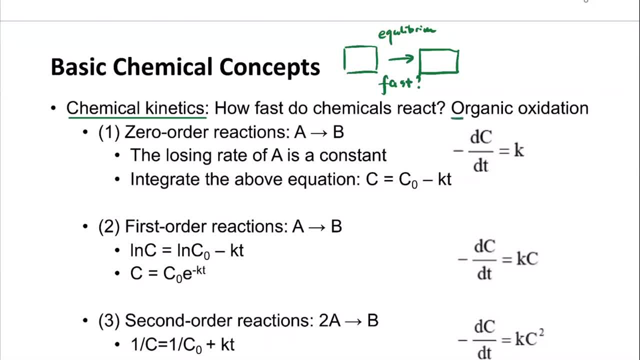 the wastewater treatment, let's say the organic oxidation. we know that in wastewater there are a lot of organics. right, we need to treat these organics, basically also oxidize them into carbon dioxide and water and water. but how fast is it going to reach the final state? okay, so this is. 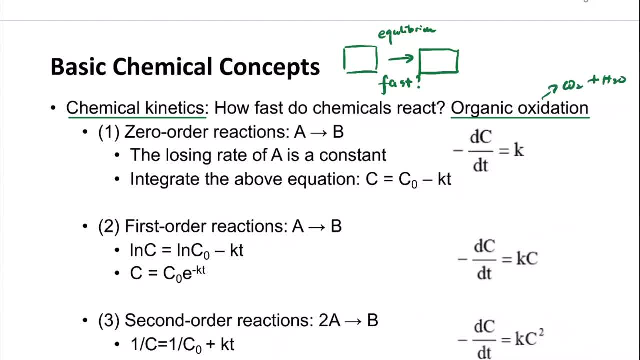 is this oxidation? is it very slow? if it's very slow, then we need to design a very large reactor and then let the water to stay there for sufficient amount of time before we discharge them into the environment. right, but if the reaction is very fast, then we know we don't need. 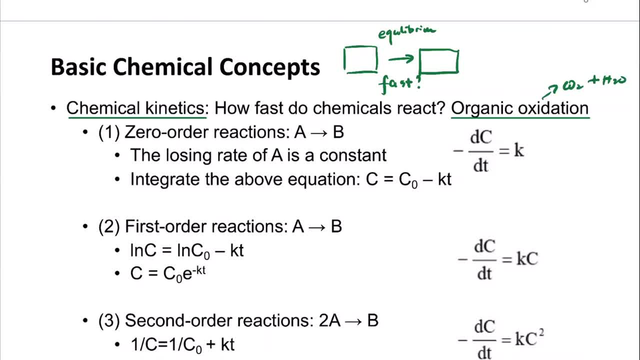 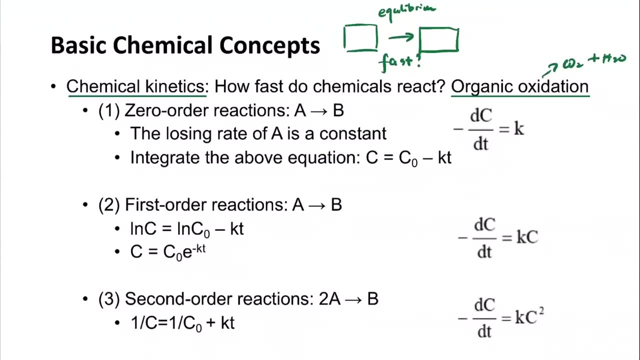 to worry about it. we can just have a smaller reactor right and then send in pretty fast or high flow rate because we know that the reaction is going to take place very rapidly, okay, so, um, because that, because of that, we need to know the chemical kinetics, and that is normally shown in. 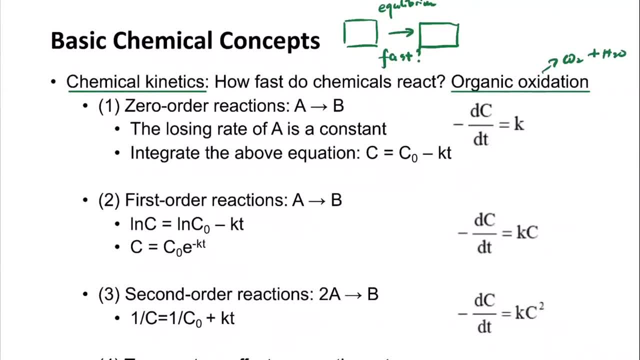 the in the reaction rates. okay, so based on the reactions, we can categorize them according to their order. okay, so we can have the zeroes order reaction, first order reaction or second order reaction. okay, so the meaning for the order here is mainly to describe how fast the reactants are. 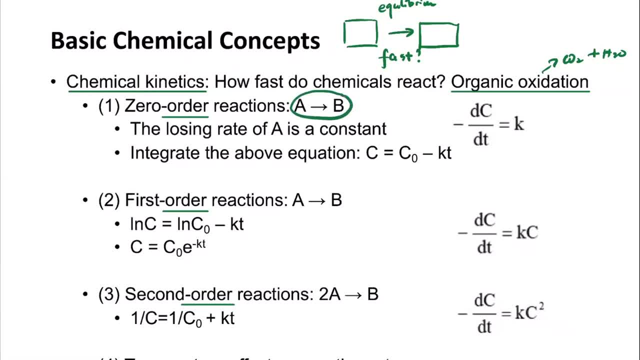 being consumed. so let's say we have a reaction of a getting converted into b. you can think of it as organic being converted into carbon dioxide. okay, so we know that the reactant concentration is always decreasing. right, so we can write out a differential term: dc- dt or dca- dt. you know that the reactant is being consumed. 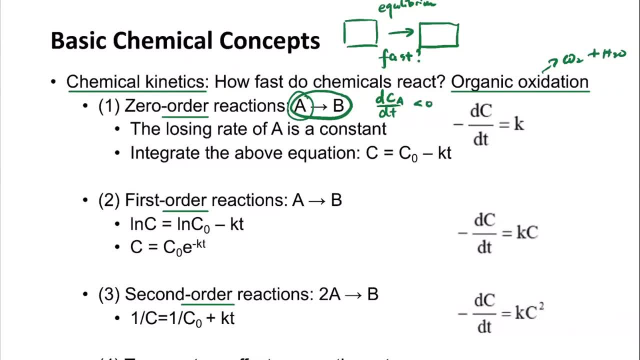 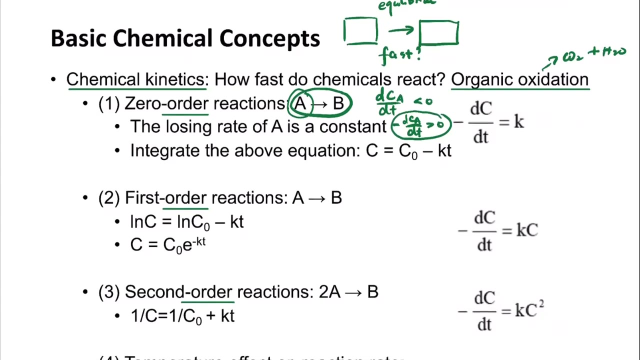 so this term is always below zero, right, it's always decreasing. so then we can write it out as dca, dt. we put a negative sign, then this is going to be positive, right, and we call this term as the reaction rate, or the losing rate of the ace of the a species. so what? the zero, zero's order, reaction. 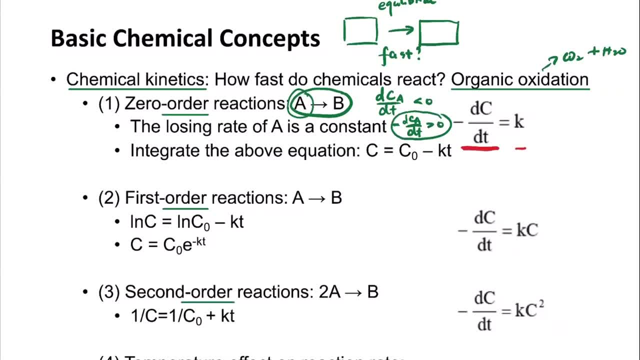 means is that this losing rate is always a constant. okay, so because of that, if we plot out the concentration of ca as a function of time, then, because it's a constant, what you are going to have is is the linear decrease of the concentration. right? so if we write out the concentration of the ca, then it's going to be c or ca equal to c. 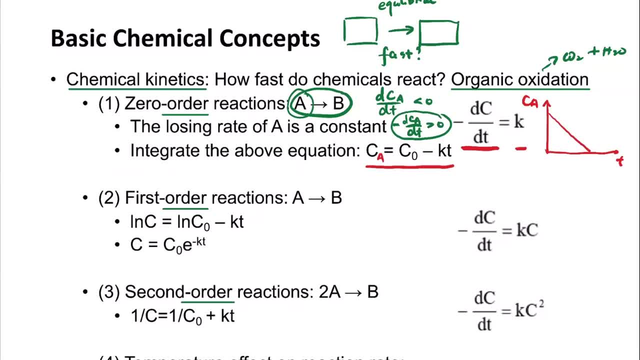 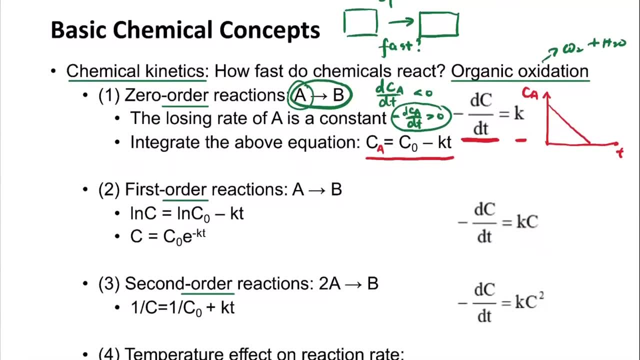 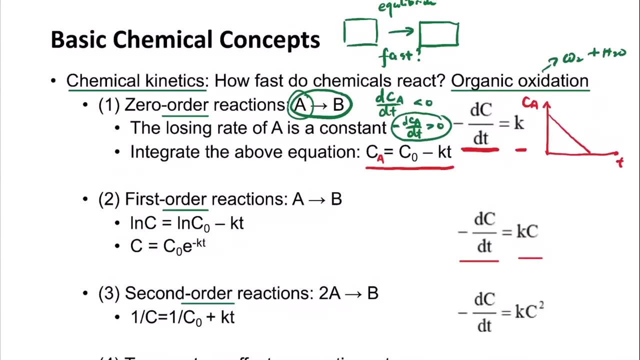 zero minus kt. so the concentration is going to decrease linearly. all right. so this is the definition of zero's order, right? and then the first order reaction means that the losing rate or the reaction rate is proportional to the concentration of the a species. actually, the first order reaction is the most common. 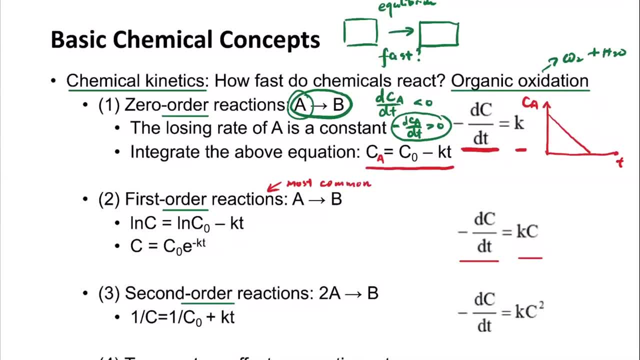 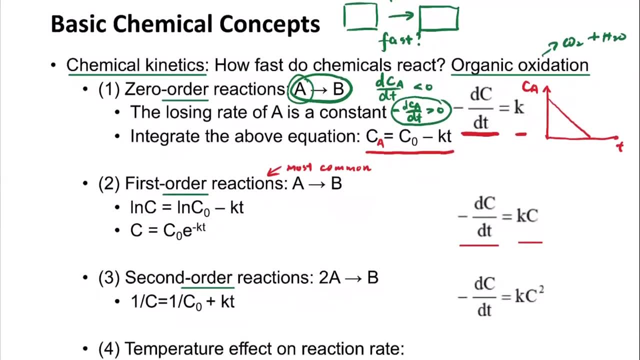 most common reaction in the environmental engineering. so we need to know this concept here. okay, so what this means is that concentration of a is going to decrease proportionally to the concentration of the a species. so what does that mean? i think from the calculus you know that we can. 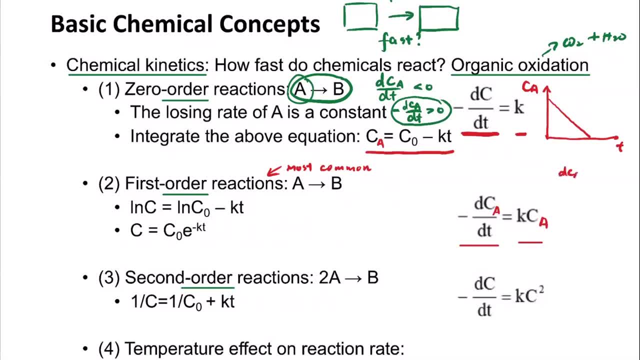 integrate this equation here. so dc a divided by c a is going to be equal to negative k dt. right? so if we do the integration, we're going to have log c a is equal to minus kt plus c. okay, so further we can solve that c a is going to be equal to c 0, exponential of negative. 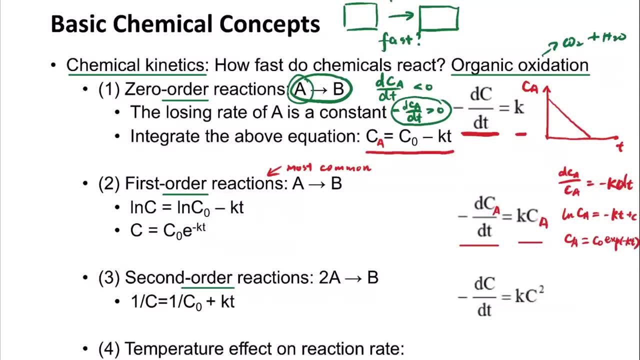 kt. okay, right. so for this concentration here, or for this reaction here, if we further plot it out, the uh, the concentration as a function of time, then it's just going to decrease exponentially. okay, so infinitely time later, the concentration of a is going to approach to zero. 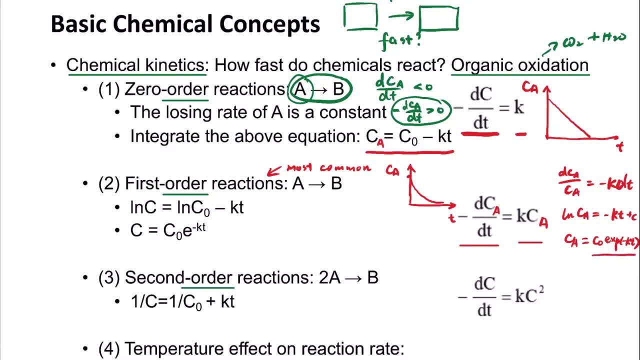 but it's not zero yet, right. so we have this exponential term here, okay. so, as i said, the first order reaction is the most common reaction in environmental engineering, because- not because the reactions are happening in this way, but because it can approximate a lot of the common reactions we see. okay. so, for example, the oxidation of the organics. 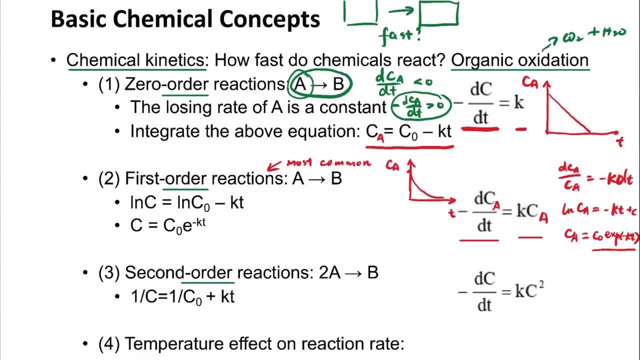 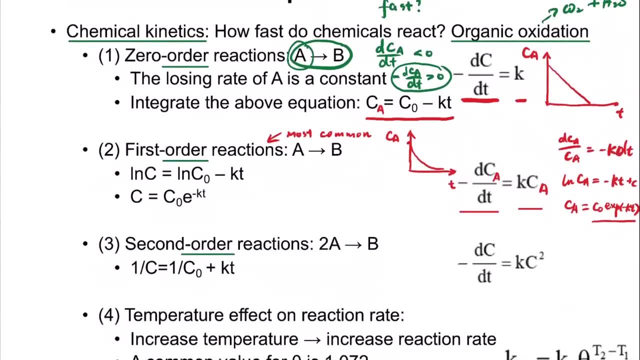 we can approximate it as a first order reaction, all right, um. so let's say, for example: okay, so, um, we're talking about the oxidation of some organic fertilizer, cool. so we're talking about the oxidation of some organic fertilizer, so fertilizer, okay. so let's say: we have the mississippi river, uh, flowing right, we have a. 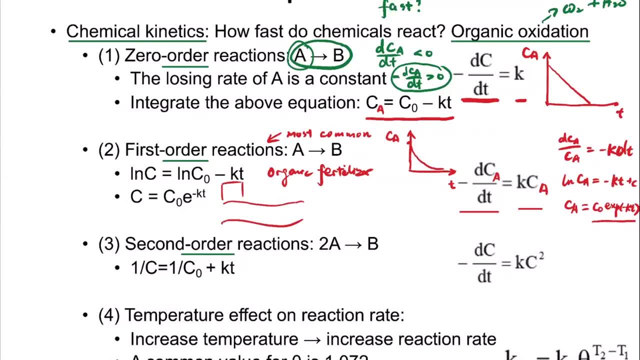 farmland in here, so we were using some fertilizer here and then the water is being discharged from this farmland and downstream of the farmland we have the city of uh, uh, st louis. okay, this is the city of saint louis and we know that the city of saint louis is mainly relying on this for uh to 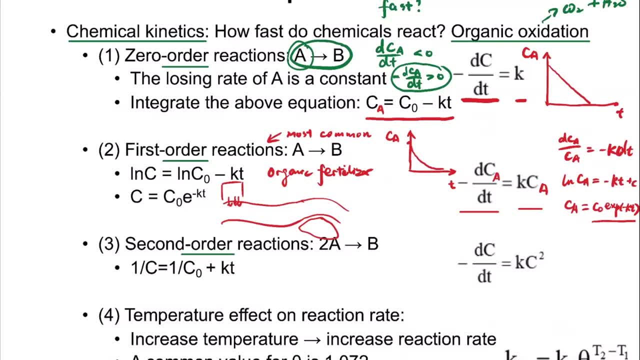 mainly rely on the Mississippi River for the drinking water. right So we have some water treatment plant to extract the water coming out of it. right So within the river there are a lot of bacteria which can oxidize these organic fertilizers into carbon dioxide and water. 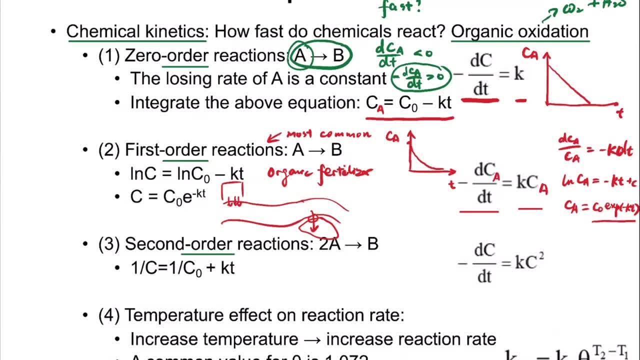 right? So definitely we don't want this water treatment plant to be very close to the farmland, because in that case we're basically human, are going to drink that, right? So under this situation, we need to know how fast this organic fertilizer being composed, right So people. 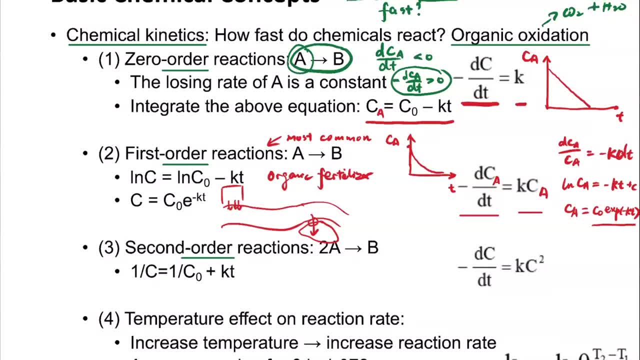 actually determine the reaction rates. They found that the oxidation follows the first order reaction And then they can also determine what is a K value. So if we find that the K is equal to one per day, okay, So it means that it reacts with a certain speed. 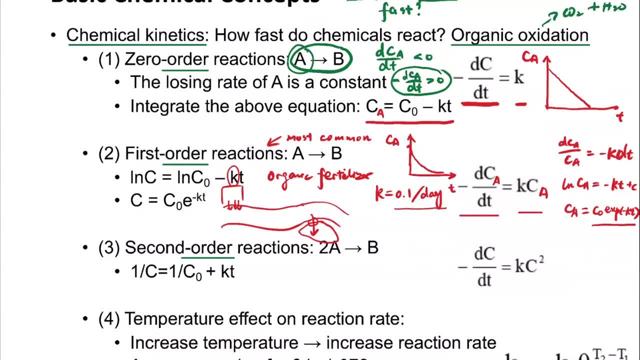 In terms of this concentration, decay, okay. So let's further assume that the concentration of this organic fertilizer is one M, okay, Or one mole per liter, okay. So we know that the concentration of this organic fertilizer is going to follow the reaction, follow the equation of: 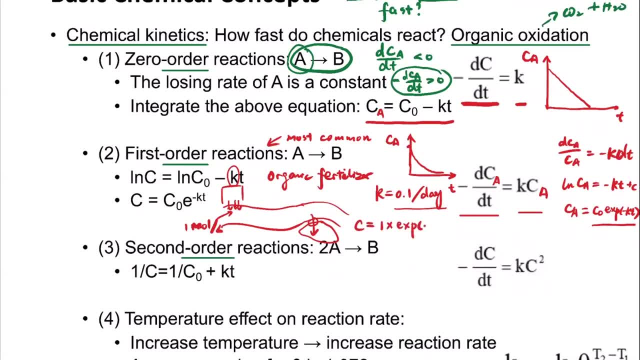 one multiplied by the exponential of negative 0.1 multiplied by T. okay, So this is basically how the concentration of the organic fertilizer is going to be. So we know that the concentration of this fertilizer is going to decay with the function of time. okay, So then we can know after. 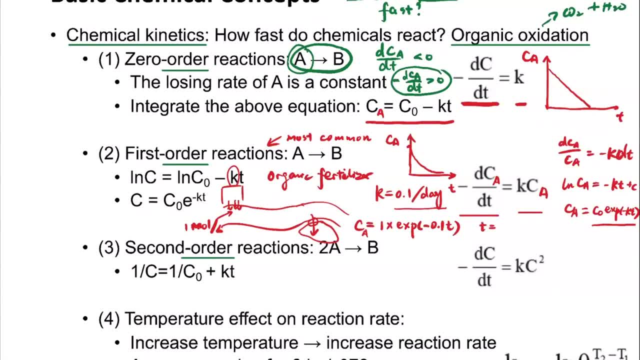 one day, let's say after, T is equal to, let's say, for simplicity, assume, after 10 days. okay, So after 10 days, then the concentration of CA is going to be just exponential of negative one. okay, So the concentration decreased, right? So then we can put these: Max and L. we will play that little bit Seek and we will see what happens, but we saw that it was fine. Okay, So this put these two together and they put up is levelts, And if you can use the same distance to the left, then you got to get the same value of value of W. 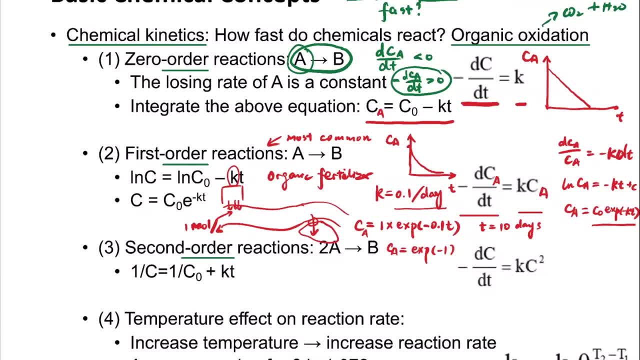 It's probably the same answer is 1 over 4.5. So this also equal. So it's going to pull in the participant. So we have a standard. I'd say instant тво is we want the concentration of this organic fertilizer to be below 0.1M. okay. So if wanted to be below point 1m, then we 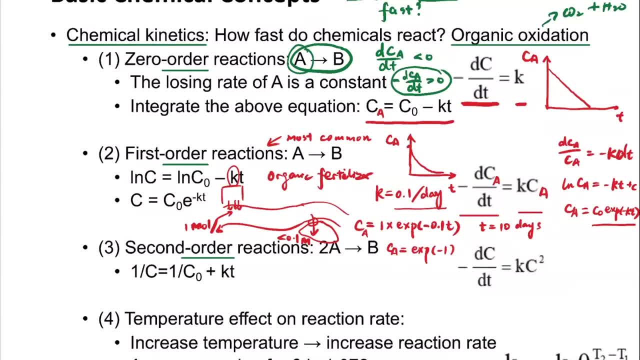 0.1m, then play in this value And then now we can plug in this valuecourse. basically, 0.1 is equal to 1 multiplied by the exponential of minus 0.1 t, So we can calculate how long it takes for this fertilizer to decay to 0.1 m. 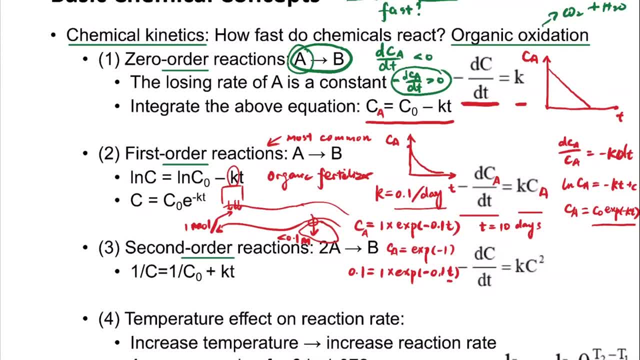 OK, so at that point we can start to extract water and send it to the water treatment plant. OK, so why is this time important? So we can. let's say we found that this time is 20 days. So if we know this time here, then further, if we make some assumption on the velocity of the river water, let's assume it's, let's say, one kilometer per day. 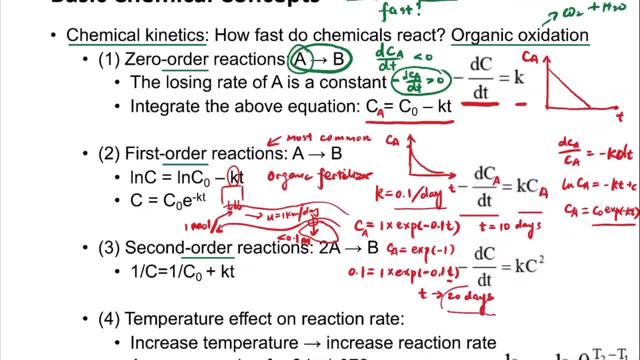 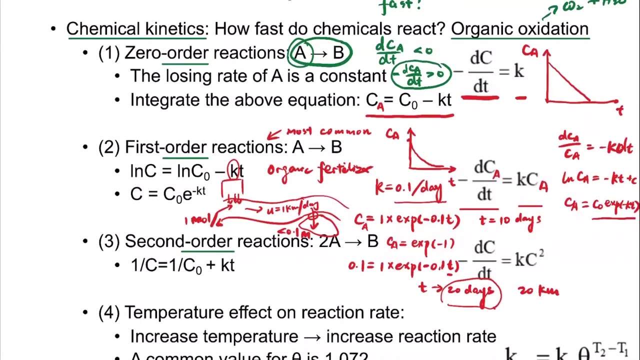 Flowing at this speed here, that if we know 20 days is the time that we need for the concentration to decay to 0.1, then we know that this water treatment plant should be 20 kilometers downstream of this farm Field, downstream of this farmland. So that's why, if we know the reaction rates, if we know the order of the reaction, 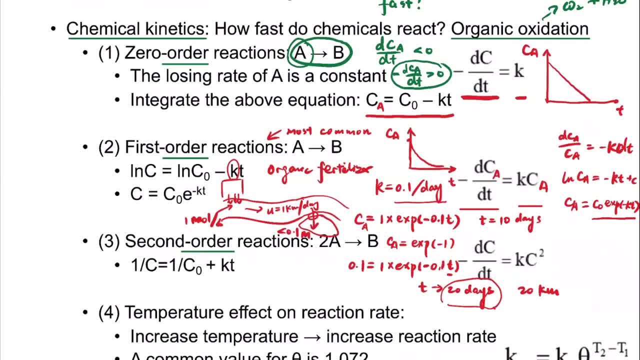 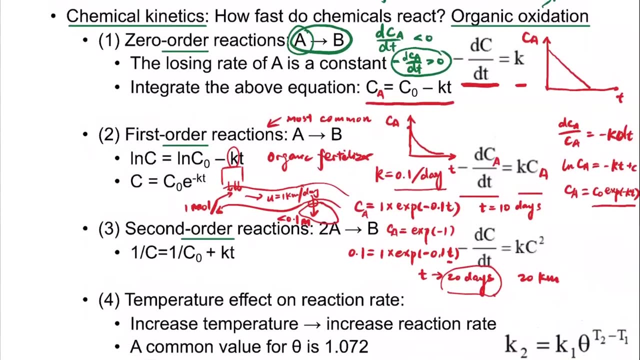 we can design a lot of systems regarding where we should discharge water or where we should extract water for these plants here. OK, so I hope this example is clear enough for you to understand the importance of the reaction rates. OK, so, similar to the definition of the zeroes. 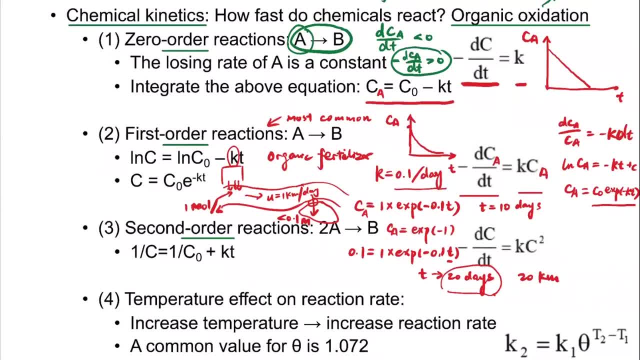 OK, so similar to the definition of the zeroes. OK, so similar to the definition of the zeroes. So in the first order first order- we can have the definition of second order, reaction, which means that in this reaction rate here I think I'm occupying too much space here- 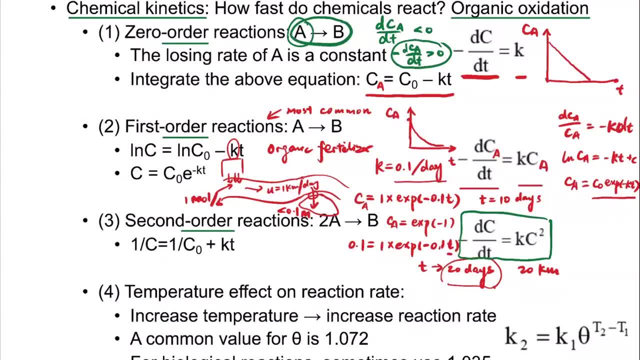 So in this reaction rate, here the reaction rate is proportional to the square of the concentration of the eight species. OK, so zeroes order means it's proportional to the concentration, to the zeroes order which is equal to one right. So the first order is proportional to the concentration of the first order. 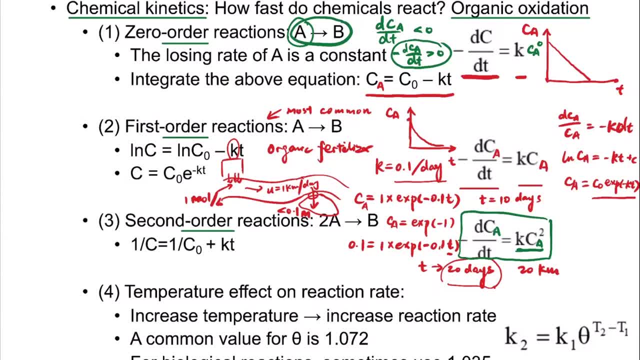 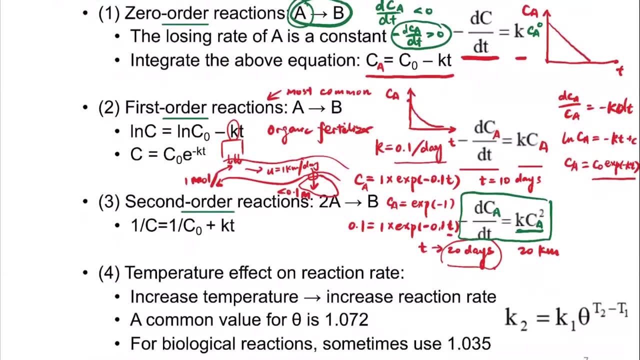 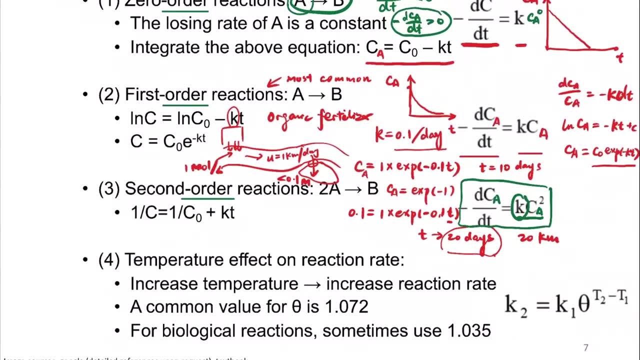 Second order is proportional to the concentration of the second order. So that's how we classify these reactions into different orders. So finally, it's some note about this K value here. So this K is defined as the rate constant, the reaction rate constant. 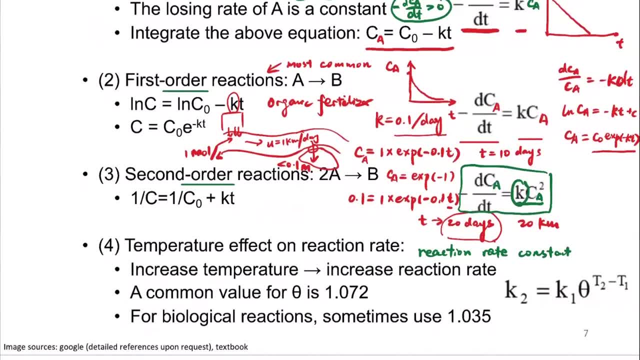 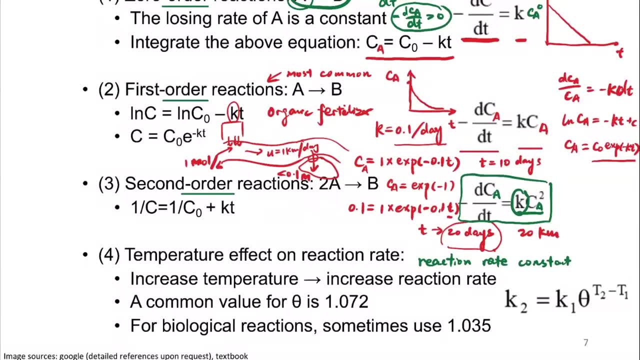 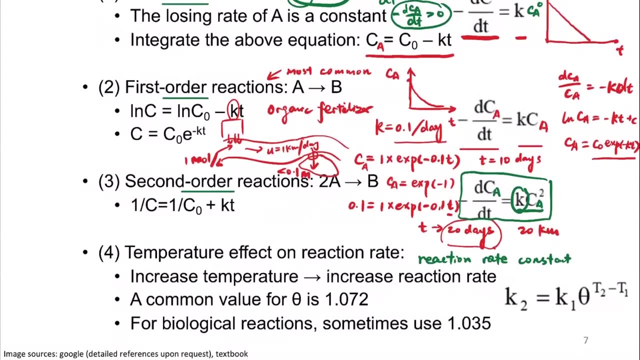 So the reaction rate constant determines what is the sensitivity to temperature. So note here that we didn't discuss anything about temperature, right? So the K here. normally it increased with temperature. So the higher the temperature, you can think of it as the higher the temperature, the faster the reaction. 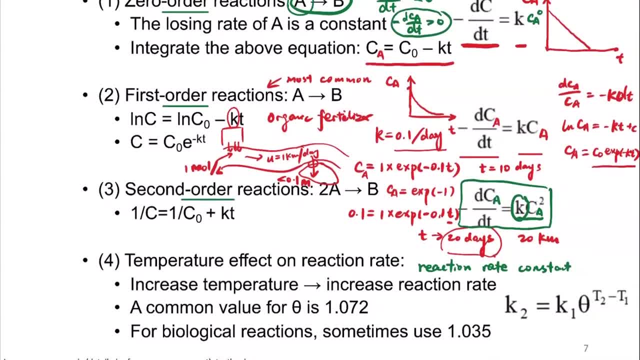 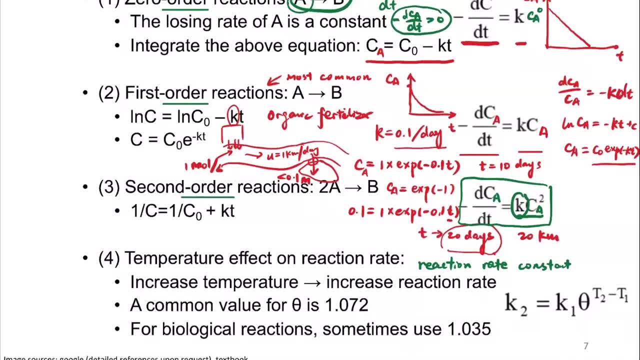 OK, but unfortunately people cannot measure the reaction rate at any temperature. So what people do is they will just measure one value, Let's say a K value at 25 Celsius. OK, so all the other temperatures are going to be interpolated from an equation that looks like this: 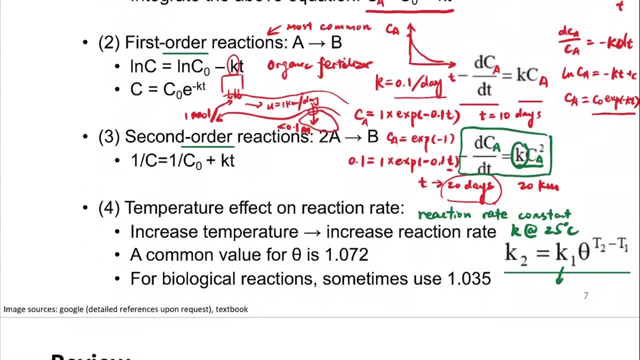 OK, so here you can think of it: K1 as the K at 25 Celsius and T1 is 25 Celsius. OK, so if we have a higher temperature- let's say very hot summer, 40 Celsius- Then if you want to determine the K2, then you just plug in the K at 25 Celsius. 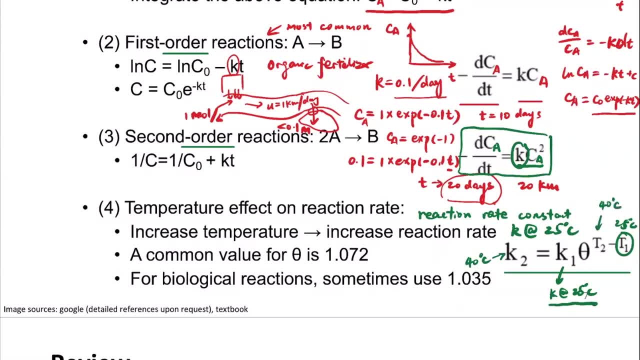 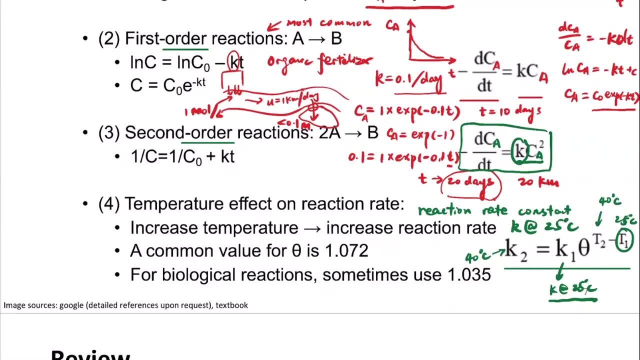 and then plug in the temperature of 40.. OK, so, as we mentioned, the higher the temperature, the larger the K. then what we know is that the theta has to be larger than one, right? Because if the theta is smaller than one, then the order of T2 minus T1, which is 15,. 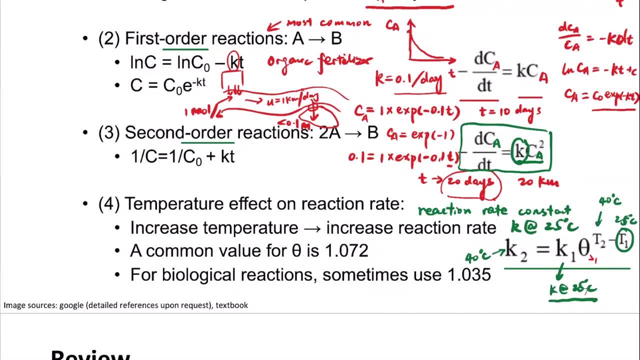 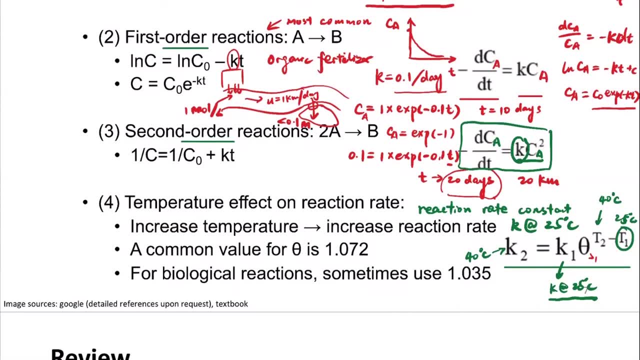 theta to the order of 15, then that's going to be a value smaller than one. What we know is that the reaction rate constant is going to increase with temperature, right, So that's why theta is always larger than one. So a common value for this theta is 1.072.. 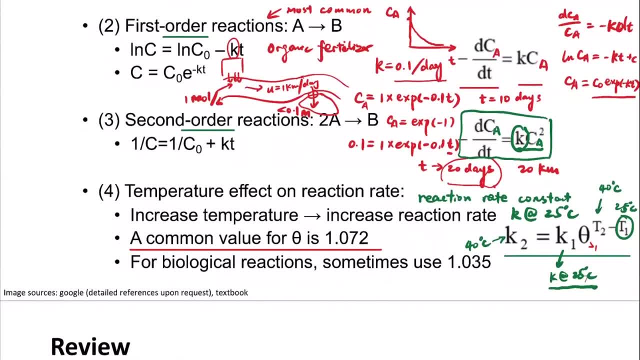 OK, so we can directly plug in this value, theta equal to 1.072. And then that to the power of 40 minus 25.. And then you can calculate what is the reaction rate constant at 40 Celsius. OK, so this is for a lot of the common reaction. 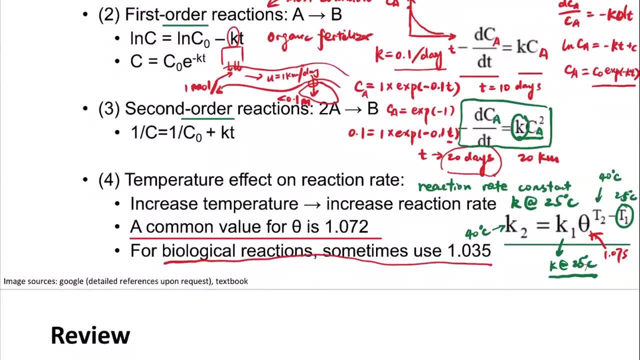 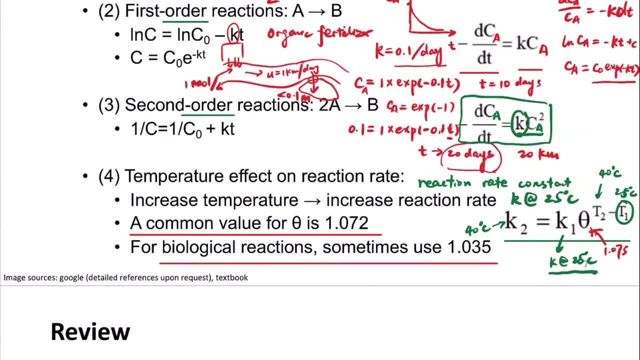 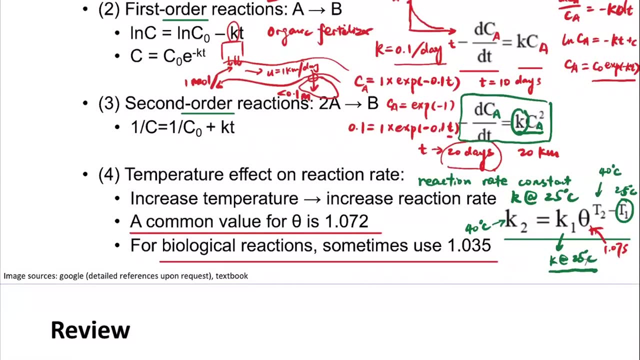 But for biological reactions, which generally happens slower people, will use the value of 1.035.. OK, so, regarding the exact values, we're going to mention them, We're going to list them in the problems. OK, so that's all for the reaction rate. 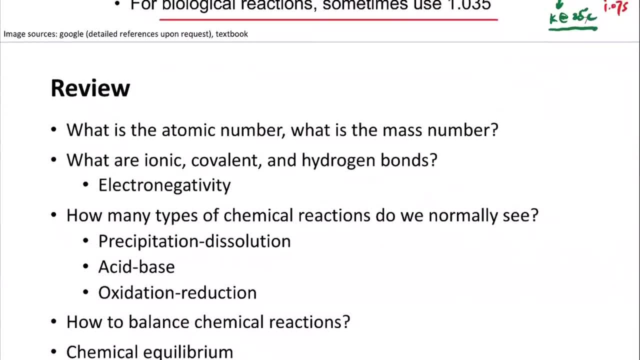 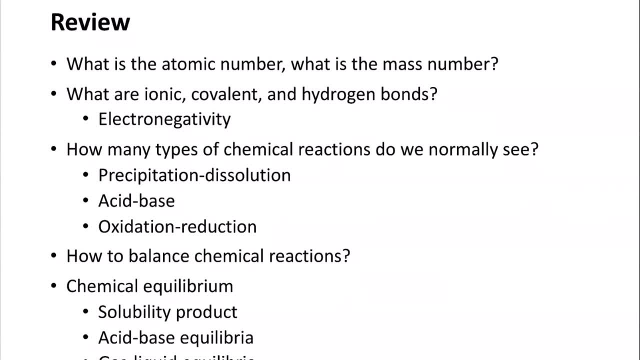 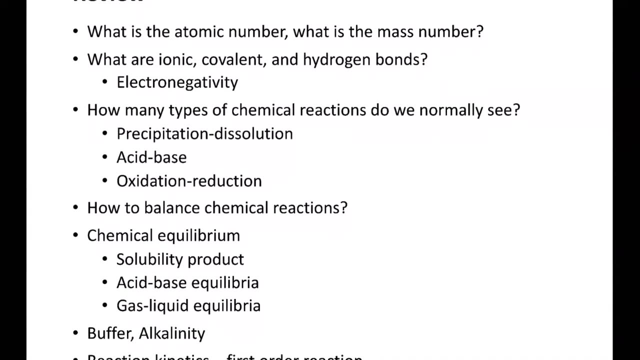 Or the reaction kinetics. OK, so now let's do a review of all the chemical principles. All right, so it took us around three classes to go over all of these concepts. OK, so we talked about what are the atomic number, What is the mass number? 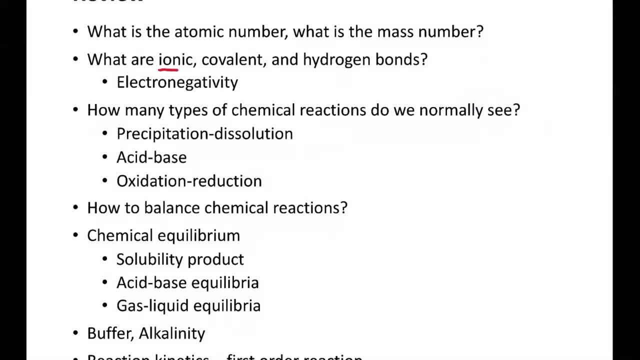 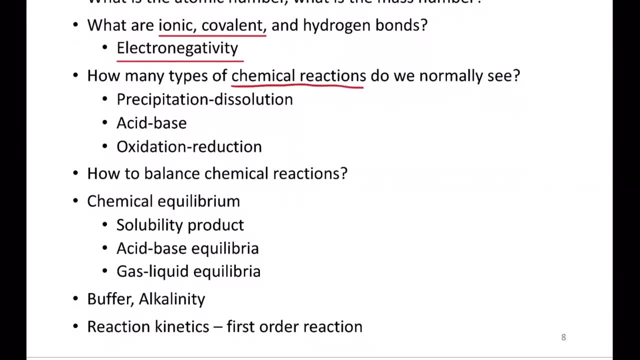 What is the atomic weight? So we introduced the ionic and covalent bonds. So the reason or the criteria to tell the difference is based on the electron, So we can calculate the difference. So we mentioned how many types of chemical reactions we normally deal with. 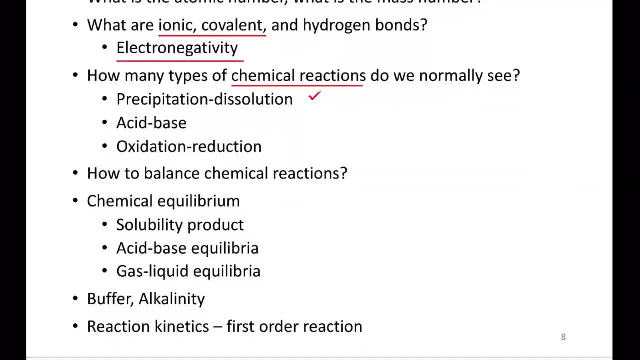 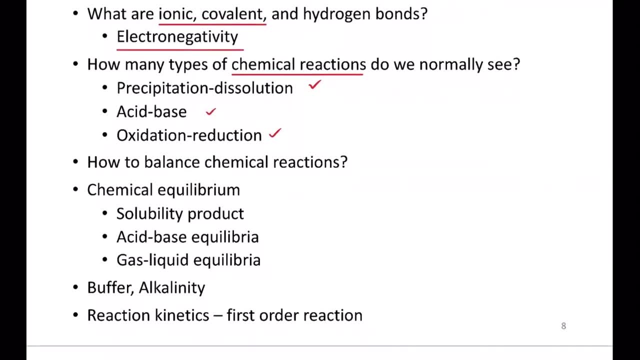 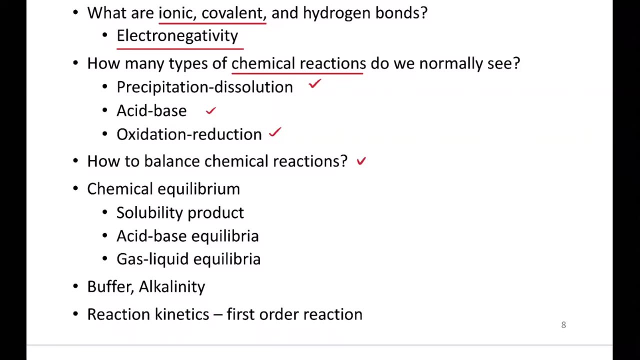 We have the precipitation dissolution reaction, the acid-base reaction and the oxidation reduction reaction. So after we introduced these reactions, we went over how to balance the reactions. We have some tricks in there to balance the reaction, because the stoichiometry is very important when we design real systems. 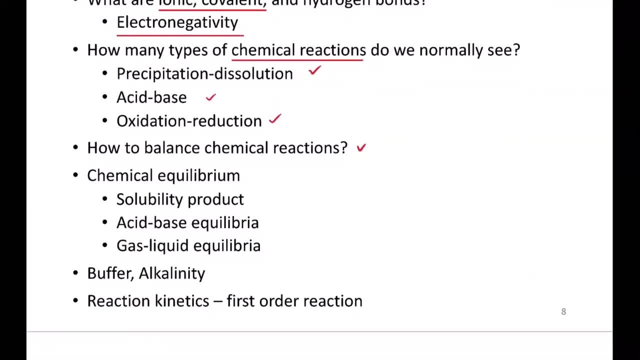 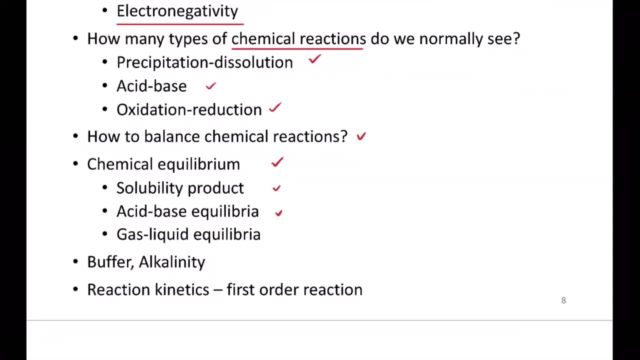 So we spent, I think, more than one class talking about the chemical equilibrium. So the chemical equilibrium can determine how much ions are being dissolved into the water from solids, It can tell whether an acid or a base is strong or weak, And it also can determine the gas-liquid equilibria. 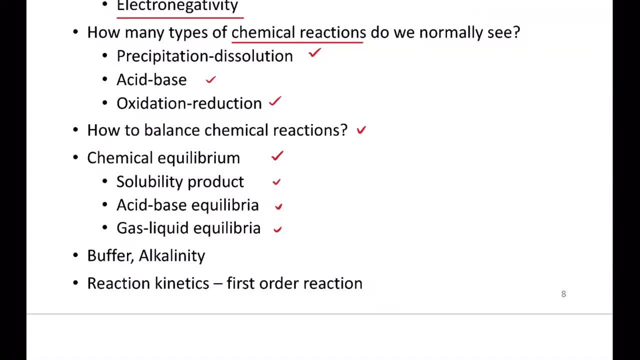 It can determine how much of the carbon dioxide can get dissolved into the water. So then, with all of these concepts, we can determine how much of the carbon dioxide can get dissolved into the water. So then, with all of these concepts, we can determine how much of the carbon dioxide can get dissolved into the water. 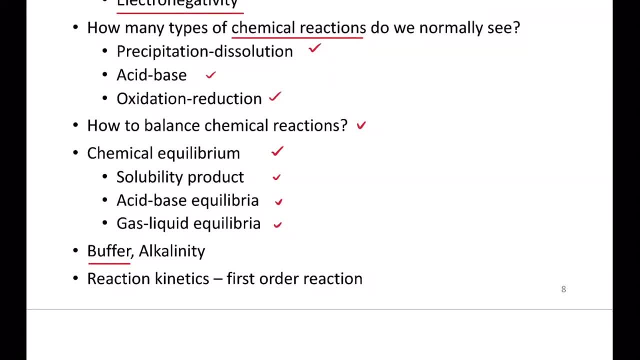 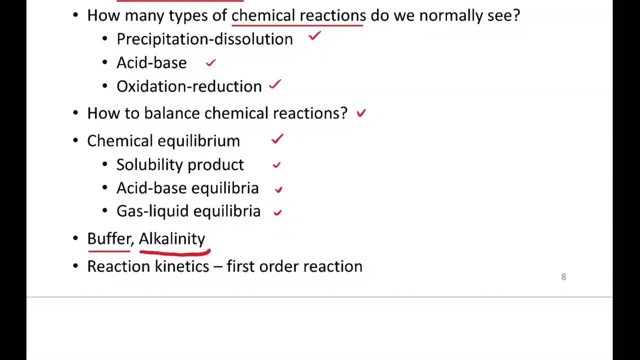 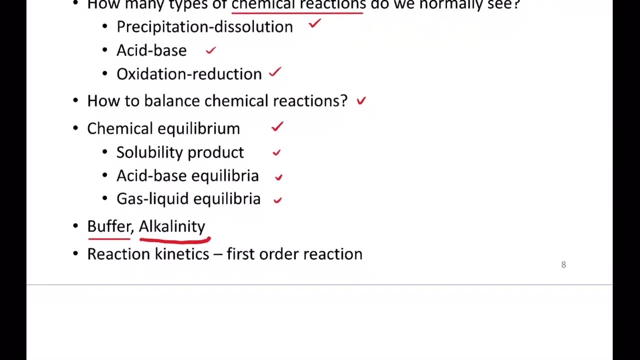 We talked about the buffer, So we solved the pH of the raindrop, And then, finally, we discussed the alkalinity, which determines basically the capacity of a solution that can react with the hydrogen ions. So at the end, just now, we talked about the reaction kinetics. 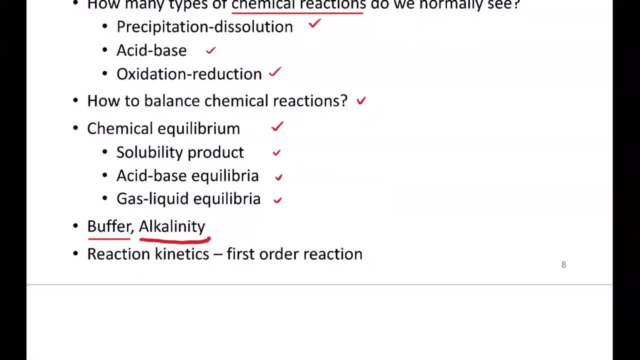 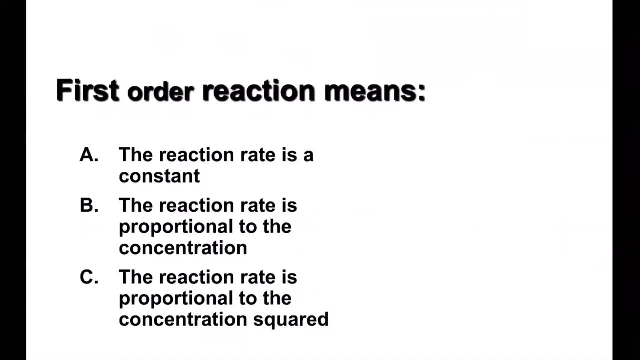 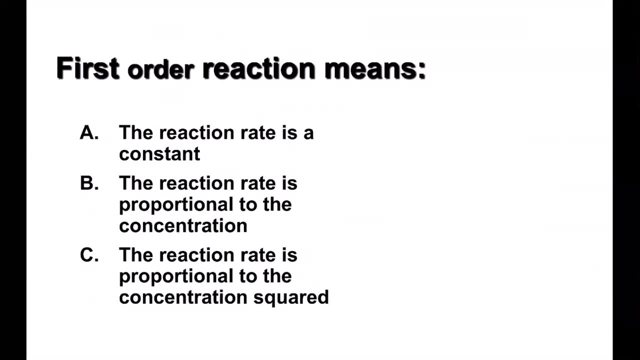 And, as I mentioned, the first-order reaction is a very important reaction in the environmental engineering. So that's all for the, the basic chemical concepts. So now let's have our second quiz here, to just make sure that you understand the questions, or you understand the concepts. 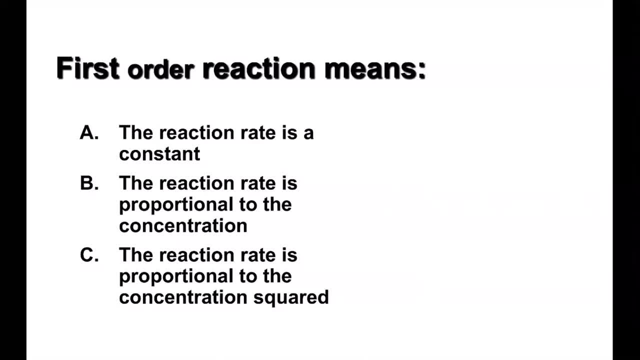 This is also a very simple question. So if we say a reaction is a first-order reaction, what does it mean? 10 seconds, 10 more seconds, All right, we'll stop here. So most of you are correct. So the first-order reaction means that the reaction rate is proportional to the concentration. 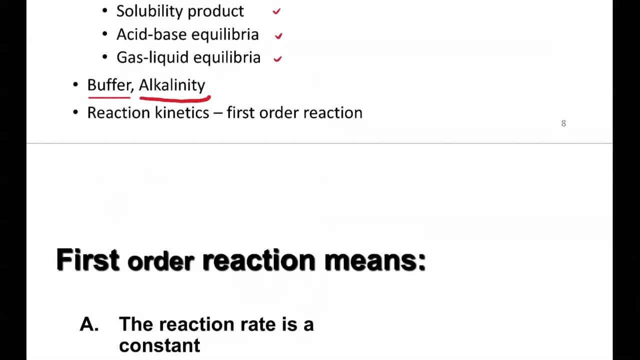 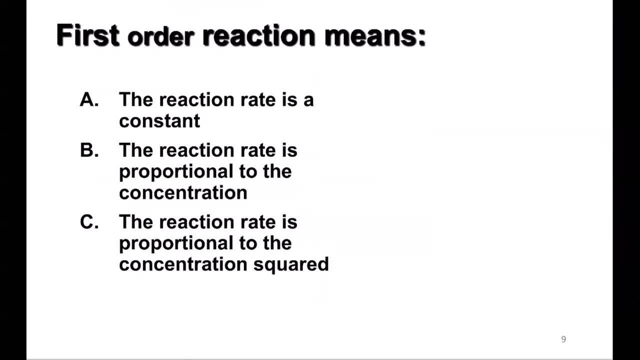 Okay, Zero order. Zero order, Okay is not dependent on the concentration right. Second order means the power of two right, So that's the definition. So if you chose the wrong answer, you can go over the contents again and then try to understand this right. 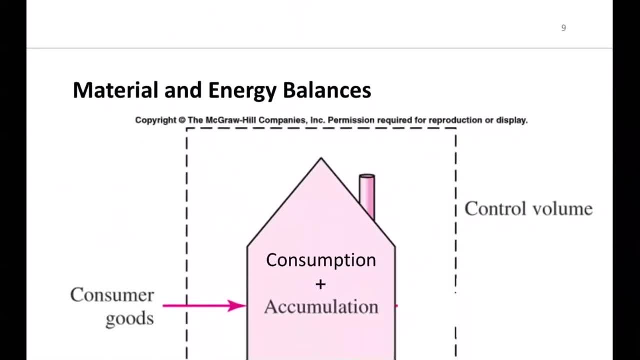 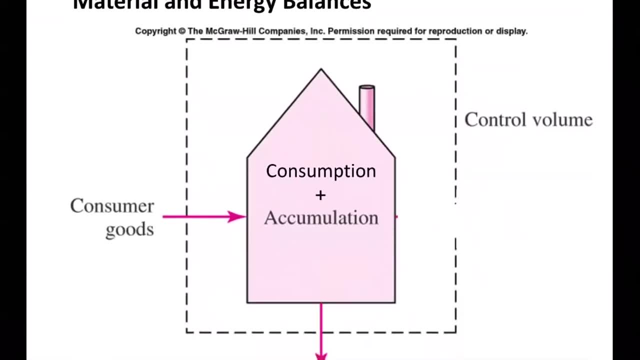 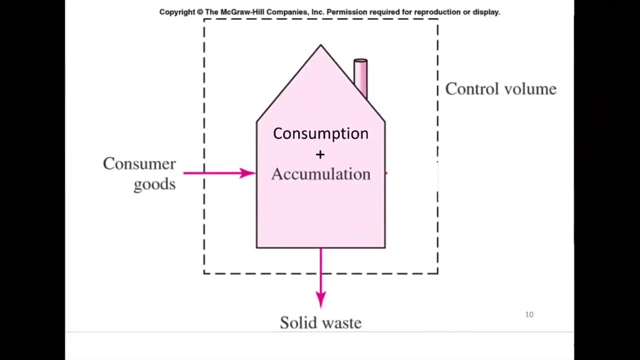 So, finally, I think we have been dragging on this basic chemical concepts for too long, So I think we can use the rest of three minutes to briefly discuss the mass balance. okay, So the mass balance basically determines what is the state of a controlled volume. okay, 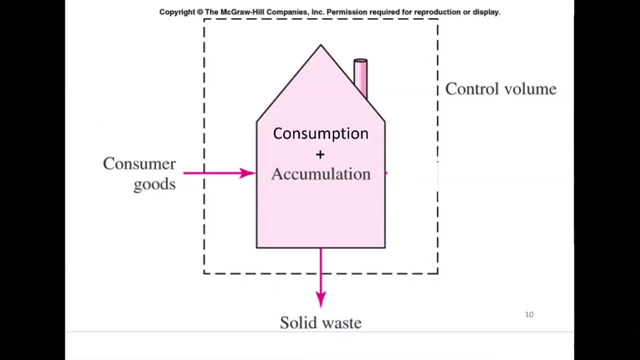 So you can think of it as going to groceries to buy, let's say, vegetables or fruits. So let's say we go to buy potatoes, okay, So I always like potatoes. I like using this as an example, also because I use that in my air pollution class as well. 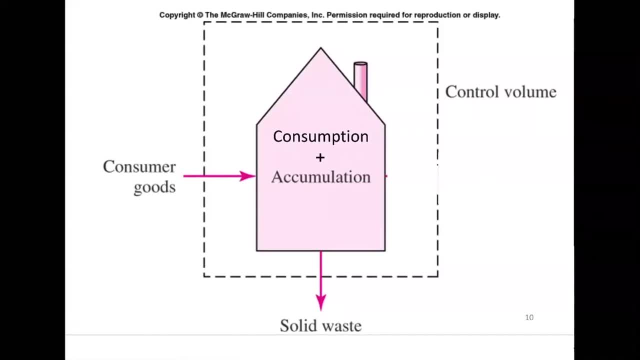 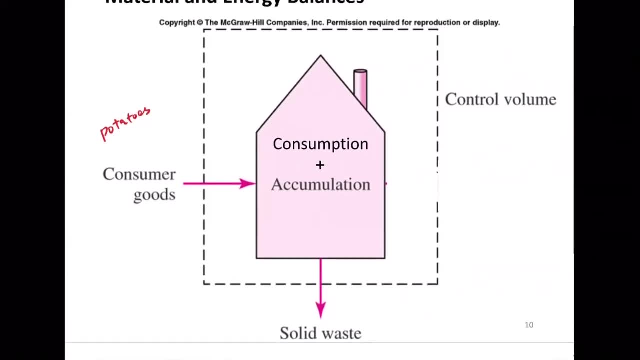 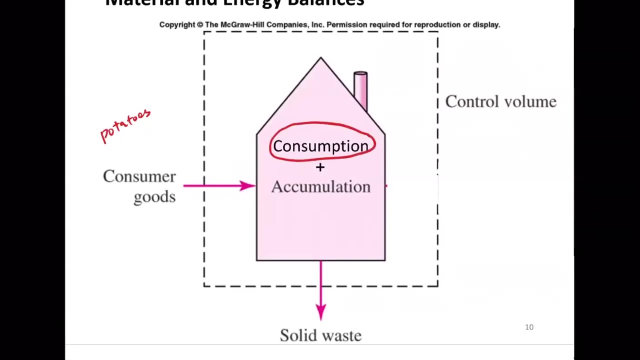 Okay, so let's say that we get potatoes, all right, So we can bring certain amount of these potatoes into our home, right? We also consume them at home and we eat them. So if you get too many, then you will place it in your fridge, right?